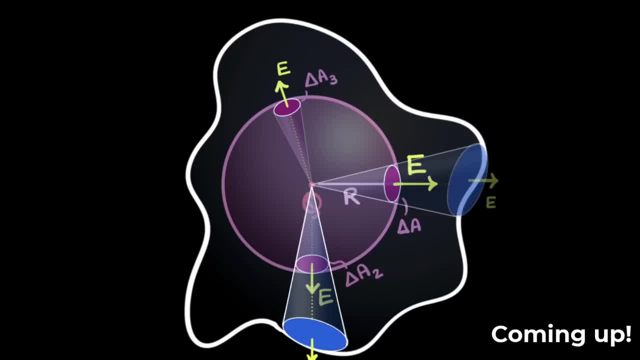 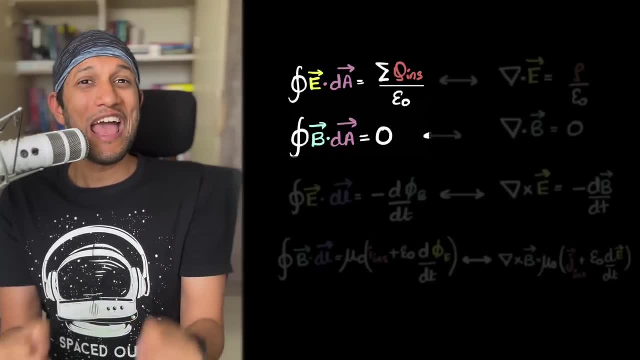 to deliver. So the goal of this video is not just to understand the Maxwell's equations- A lot of videos does this- but instead it's to get a much deeper understanding of the first two equations. We'll focus only on the first two and use it to solve the problem that Newton couldn't for years. 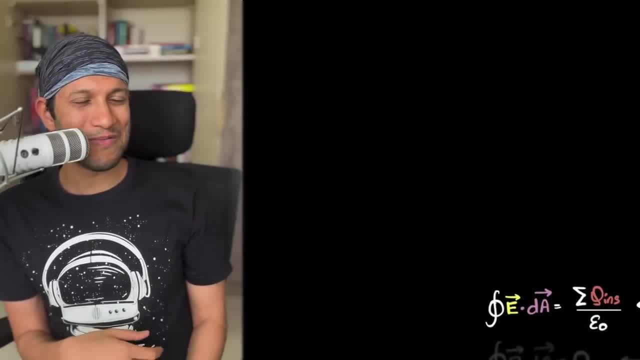 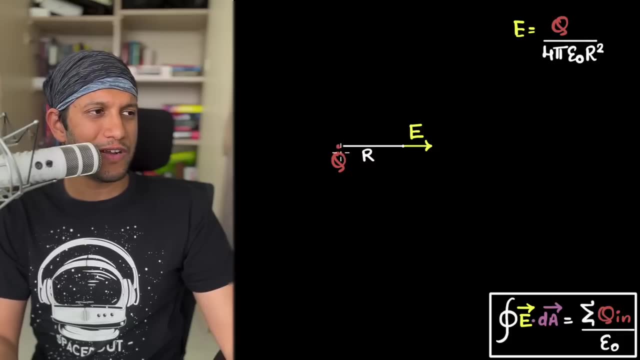 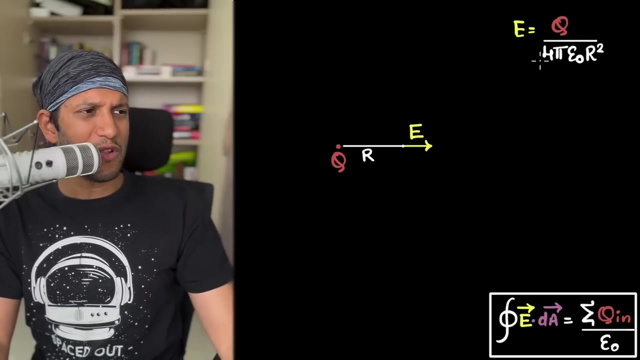 So if you're ready for it, let's begin. Let's start with Maxwell's first equation. So we start with Coulomb's law. It says that if the electric field at some distance are from a point, charge will always equal q divided by 4, pi, epsilon, not r squared, The inverse square law. And Feynman says: 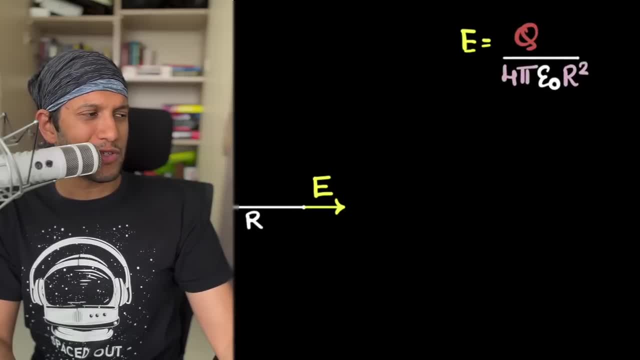 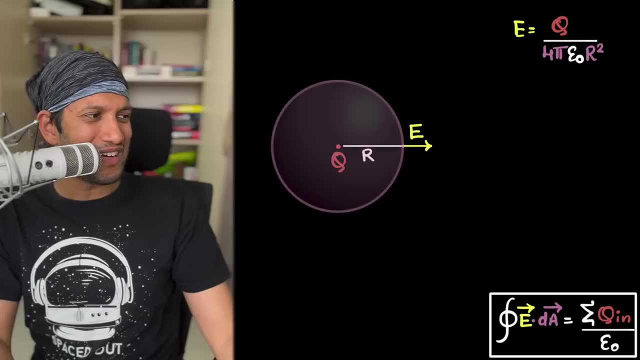 look at the denominator Mahesh. Do you see a 4 pi r squared? Do you know what that is? And I say yes, I know that 4 pi r squared is the area of a sphere. It's going to be the area of this sphere. 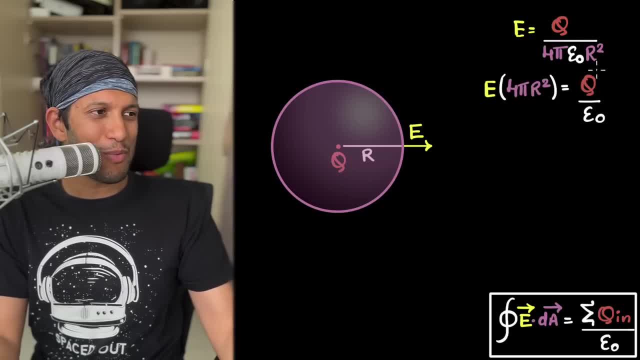 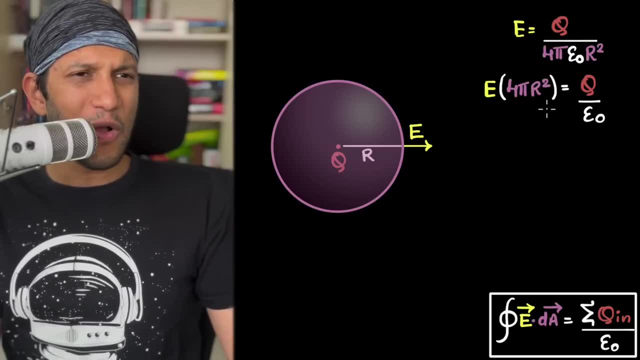 And so then we rearrange it to get this equation, We bring that 4 pi r squared on the left hand side and look, we already kind of sort of have a skeleton of our eventual law. Feynman says: this is already a more elegant version of this, and I'm like: wait a second, how is this more elegant? We just 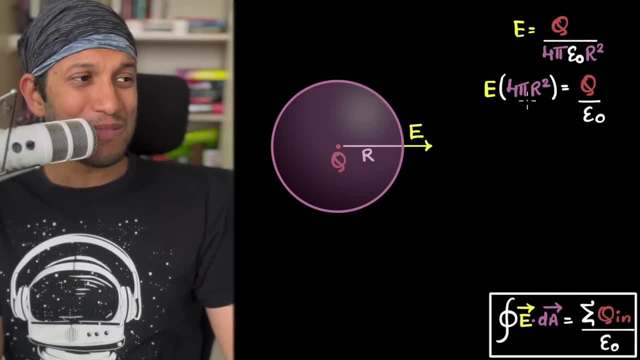 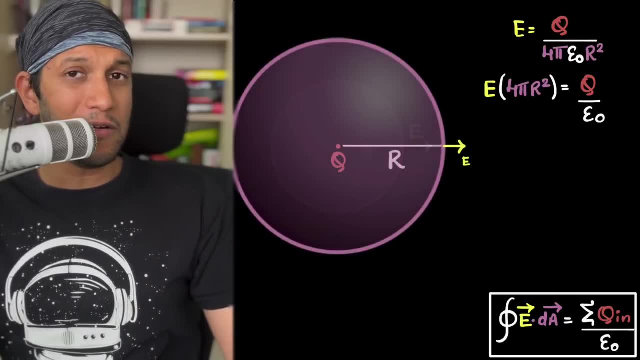 rearranged it right. So he says: look, this product, whatever that is, is a constant. It does not depend upon the size of the product. It does not depend upon the size of the product, It does not depend upon the size of the sphere. Look, if I make that sphere bigger or smaller, I will get the same answer. 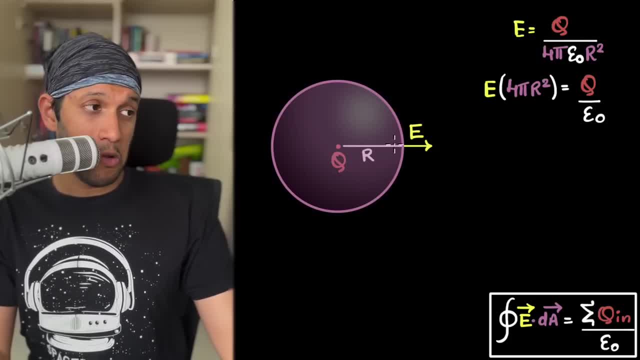 q divided by epsilon, not? And I say, okay, but what exactly is this product? I mean, multiplying electric field with the area of a sphere. sounds so random. Well, he says that, Mahesh, maybe that's not what we are doing. Probably what we're really doing is you're multiplying electric field with a. 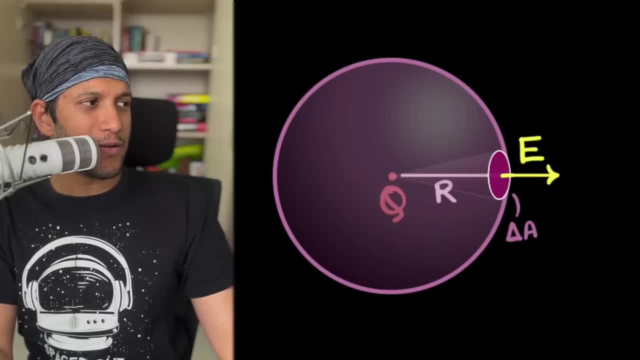 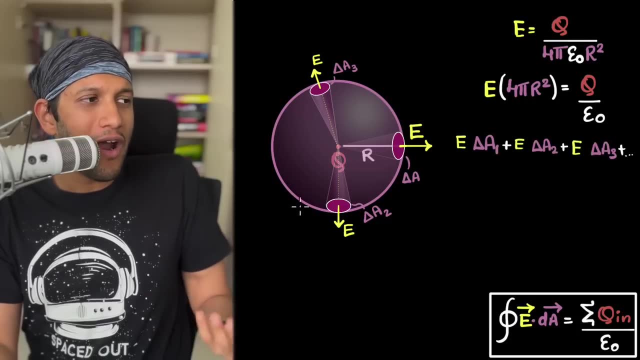 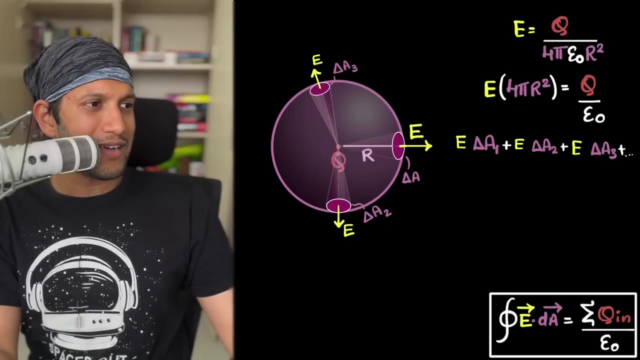 tiny local area at that point, And then we're doing it over the entire sphere and we're just adding them all up. It just so happens. for our case, electric field is the same everywhere on the sphere because the distance is the same And therefore in our case, electric field pops out. 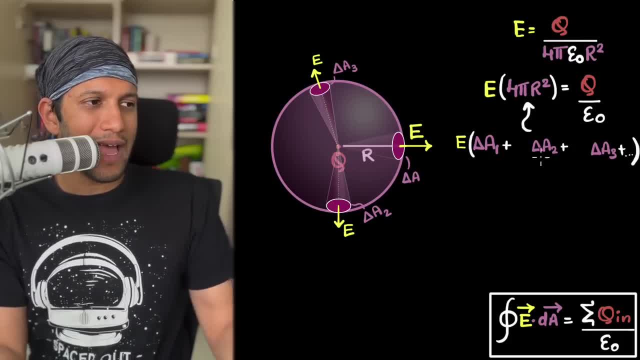 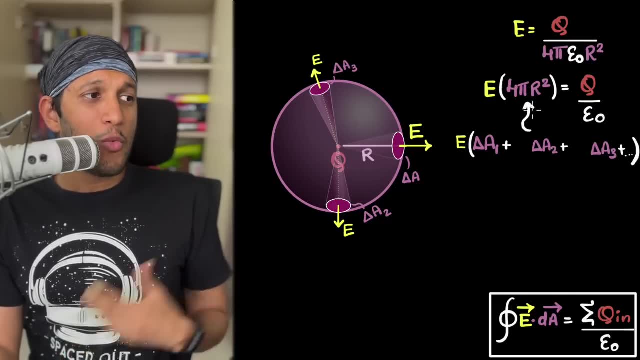 of that summation and that thing in the bracket just adds up to give you the total area of the sphere. right, If you take, adds up, if you add up all the tiny pieces, you get the area of the sphere, which means in reality what's happening, what we are really doing. we are doing a summation of 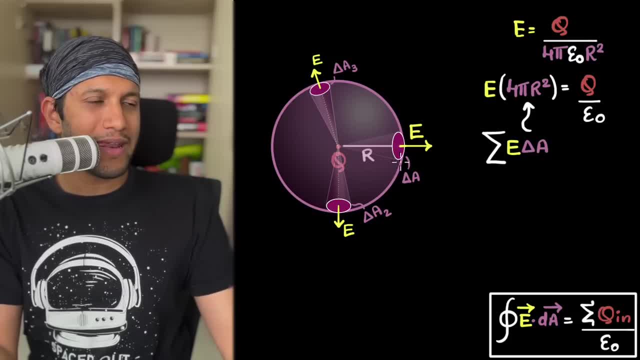 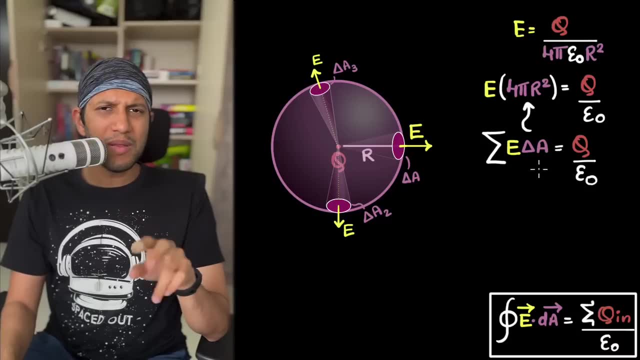 electric field and the tiny local area at n. So we're just adding them all up and we're just everywhere and adding them up, And that is equal to q divided by epsilon, not- And at this point I say: well, wait a second, Feynman, what do you mean by? let's generalize this, Because this only works. 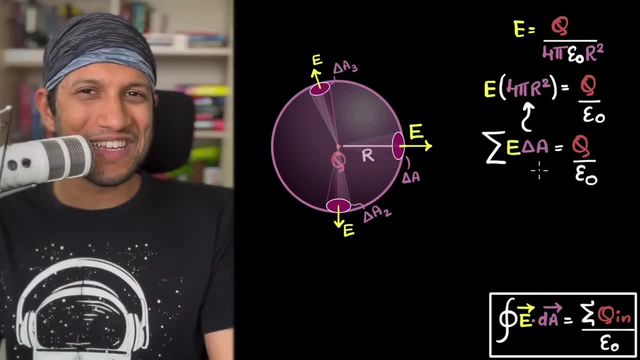 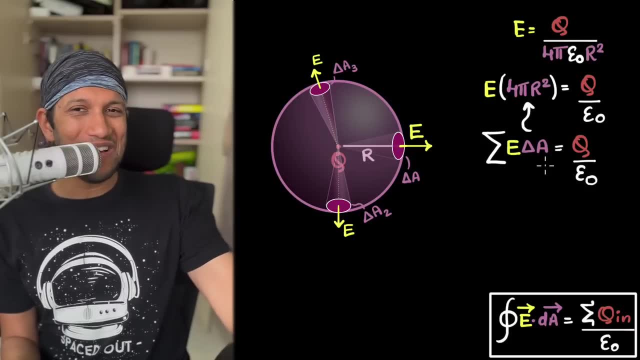 for a sphere, isn't it? And this is where he smiles and says: no, Mahesh, this will work for any shape. What We just derived it for a sphere. We looked at the area of the sphere, Feynman, How can you say? 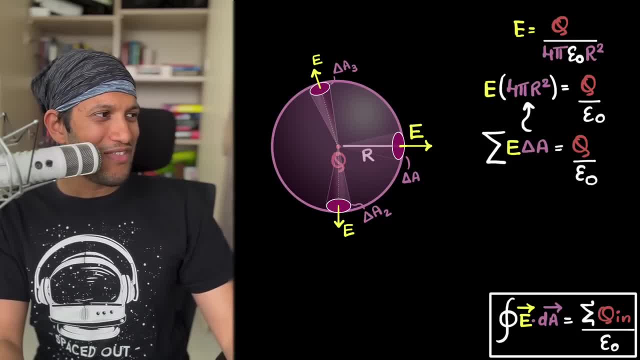 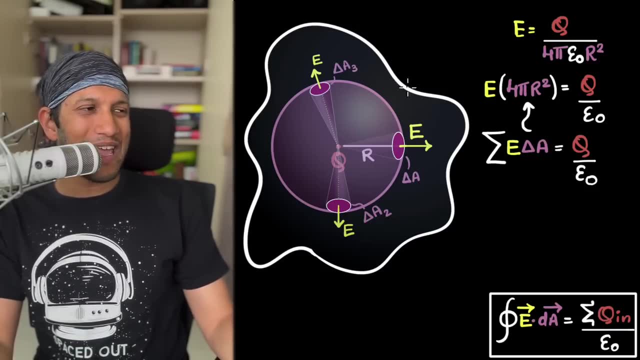 that this works for any shape. So, Feynman, are you saying that if I take some random close shape and if I take the electric field at any, every point multiplied with the tiny area and then add it all up, I would still get e times 4 pi r squared? Feynman says: yes, I am. 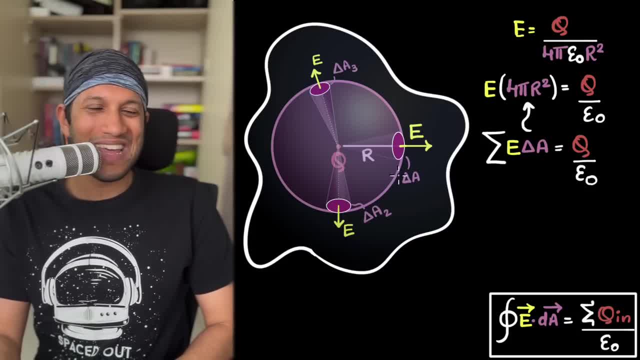 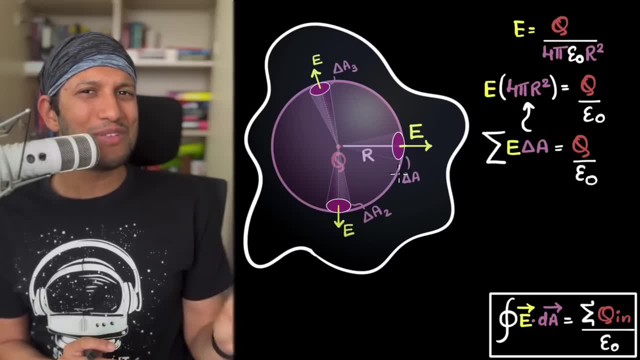 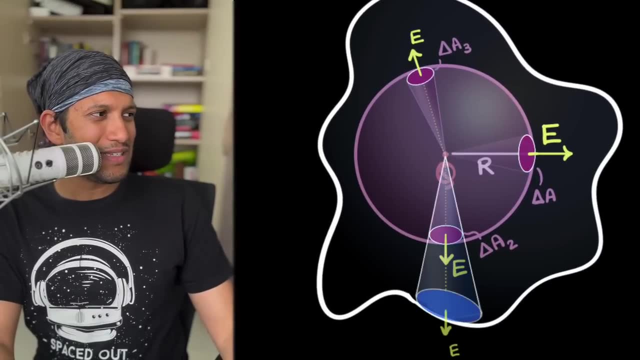 intrigued Feynman: How do you say that? And this was, by the way, one of the things that I felt like. not many textbooks explained it, But Feynman's argument is beautiful. So how does he go about it? Feynman says: let's consider a tiny piece. 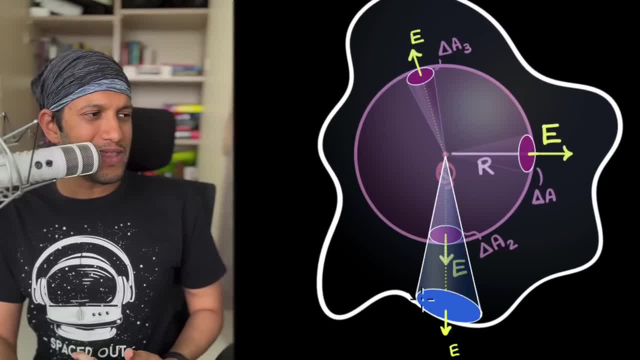 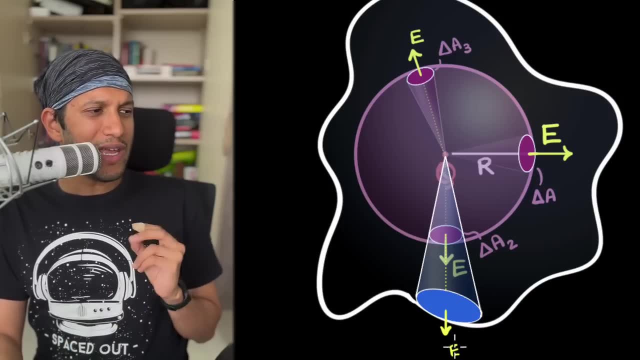 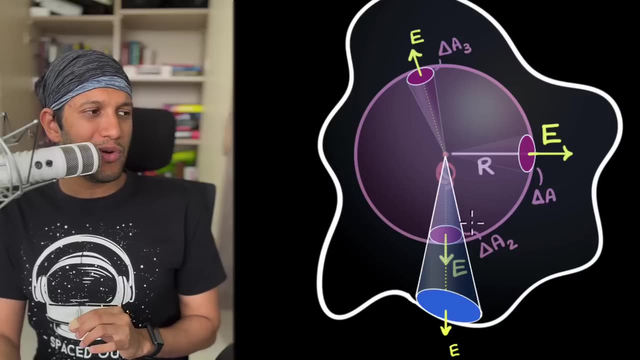 On the big area, big surface that you have drawn such a way that it sort of forms a cone with this piece over here with the charge at the apex. Now he argues that if we can prove that the electric field here multiplied by the area here, if that product equals the product over here. 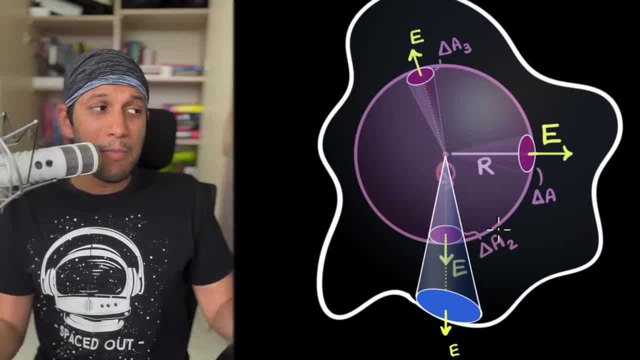 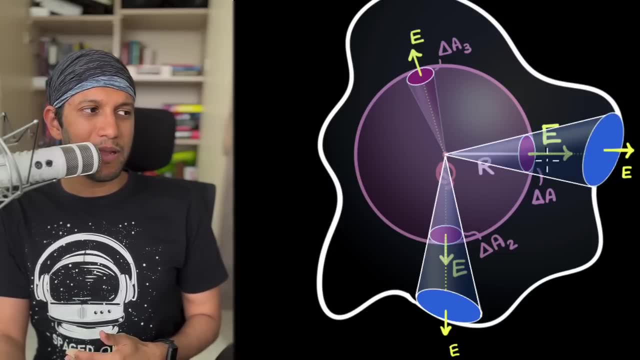 electric field multiplied by the area over here, then we are done, Because then we can prove the same thing with the same argument, that here the product should be equal to the electric field multiplied by the area here. So we can prove that the product should be equal to the electric field. 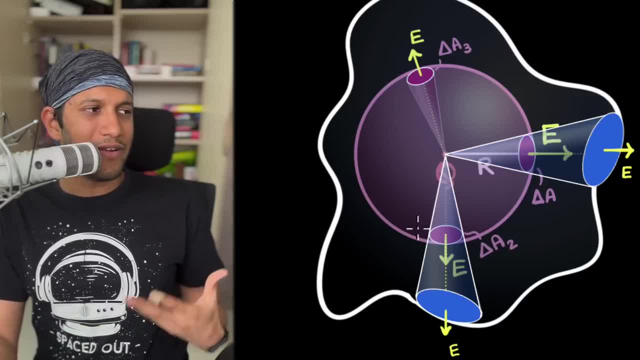 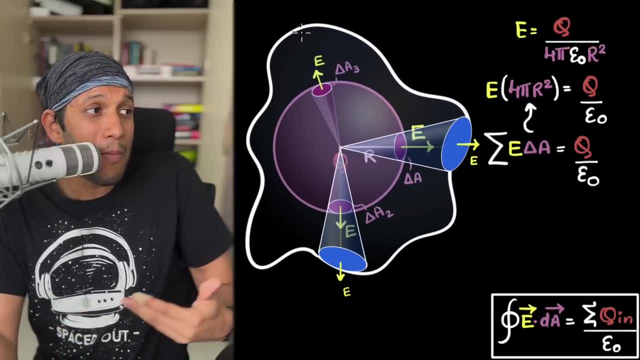 multiplied by the area here. And then we can do that over the entire case, entire surface, and prove that the electric field multiplied by the area is equal to the corresponding piece here. which means, if you sum up the electric field multiplied by the area here, that should be the same as the summation. 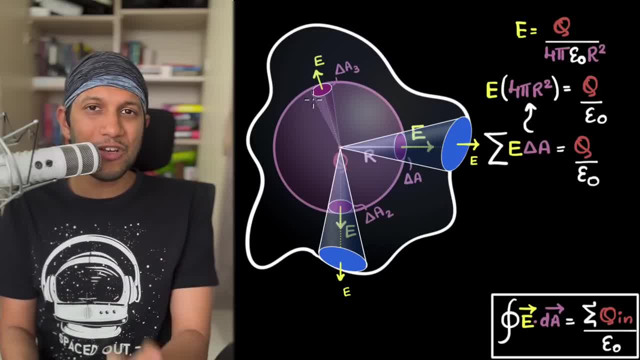 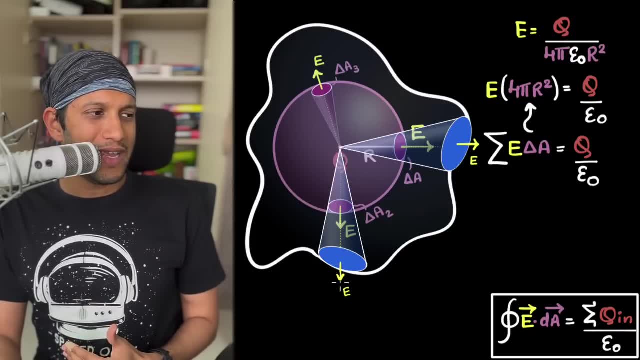 of the electric field multiplied by the area here. That's the central argument that Feynman is doing. Just to be clear, what he's saying is that all we have to do is prove that e to delta a here is the same as the e to delta a here. 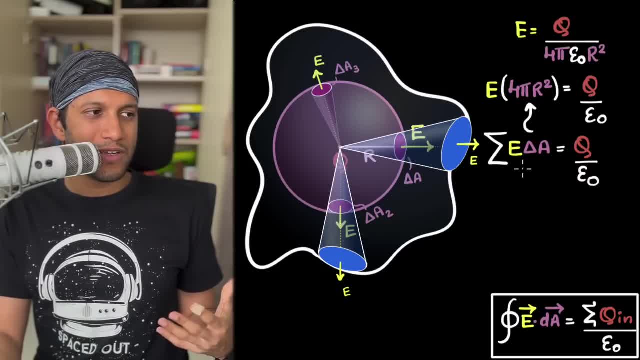 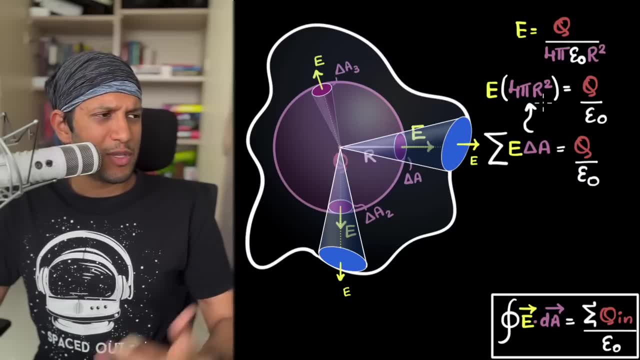 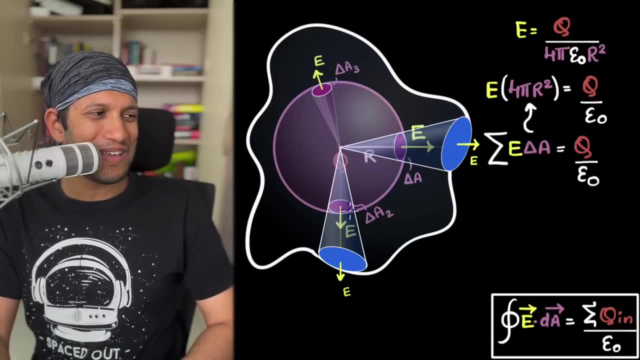 Then we can do it everywhere, and then we can say that this works in general. For any shape, this will yield the same result, And I'm intrigued because we've taken a random shape. Feynman, how in the world are you going to prove that the e dot e times delta a here is the same as the e times delta a? 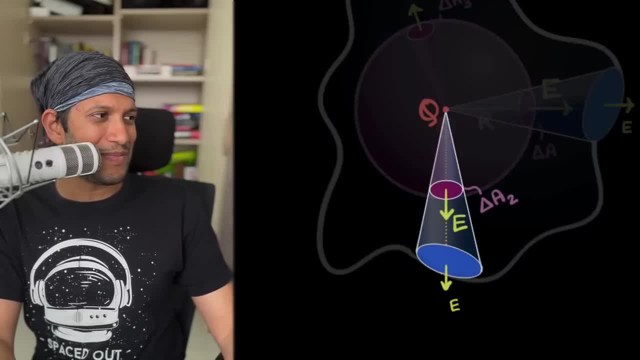 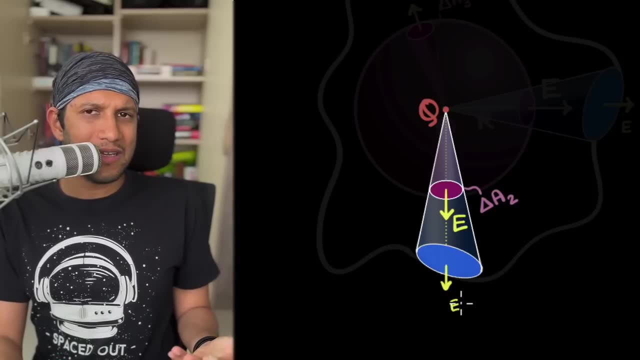 here. Well, he says, let's do that, Let's concentrate. He asks me: well, Mahesh, what is the electric field here compared to here? I tell him that it's smaller, but I don't know how much it is. He has asked us to assume something. Let's say that this distance, this big distance is. let's say: 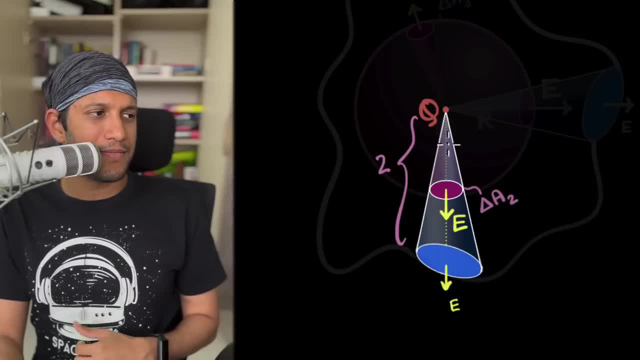 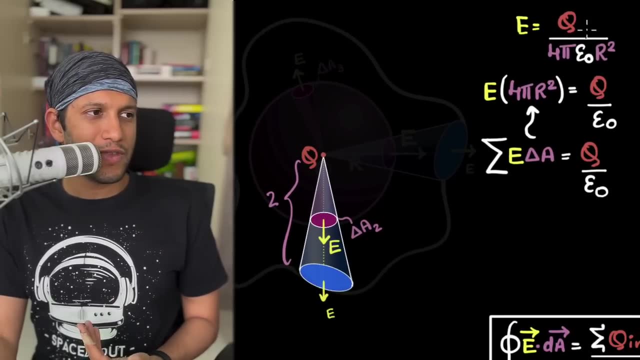 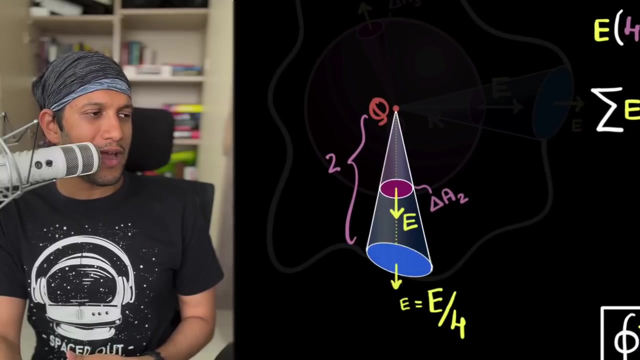 twice as much as this small distance, the radius of the sphere. Okay, now how much is the electric field? Well, if you go twice as far from the charge, then because of the inverse square law, you get a, two, r in the denominator, you get four, and so the electric field goes down as one over four, and so 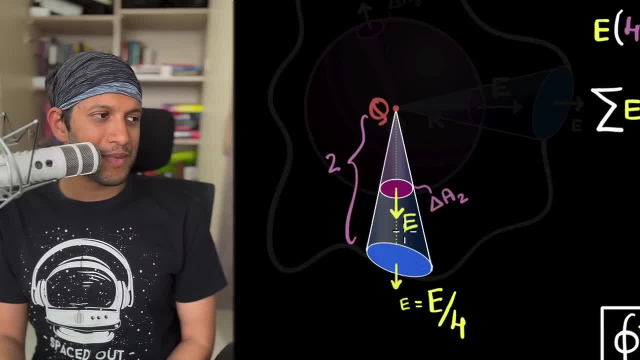 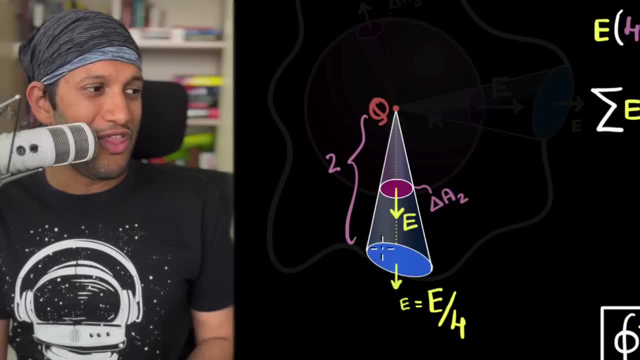 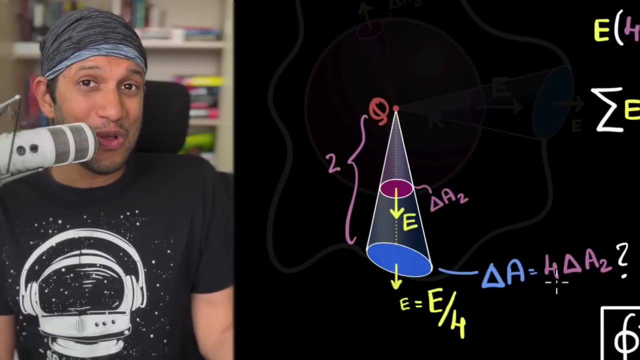 this electric field is one fourth of this electric field, which means, I mean it's saying that all we have to check now is if this area is four times as big as this area, Because then if this is true, we're done, Because the field has become one fourth area has become. 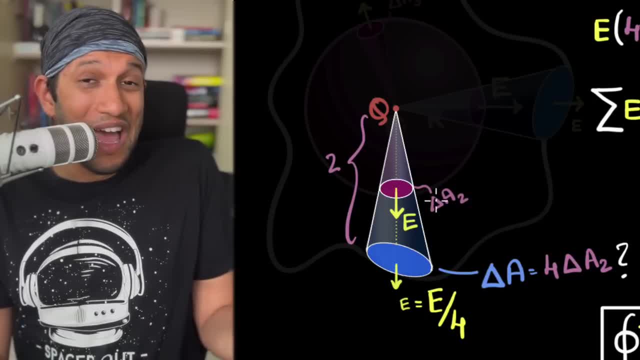 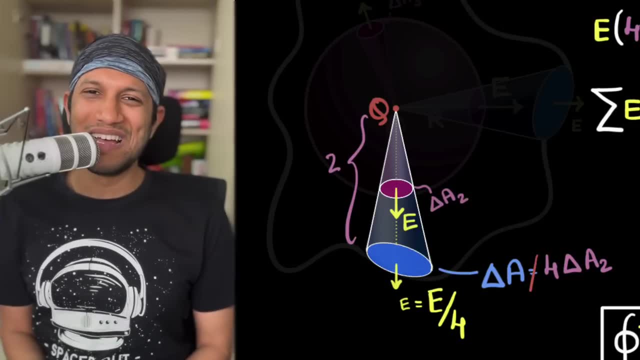 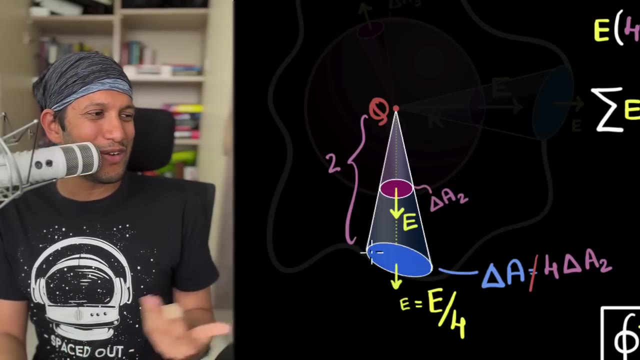 four times more. so the product will be exactly the same as the product here, And so the question is: will this area be four times as much as this area? and Feynman says no, it won't be. I mean, how can it be? it's a random piece that we have chosen. look at it. it's not even forming a right circular. 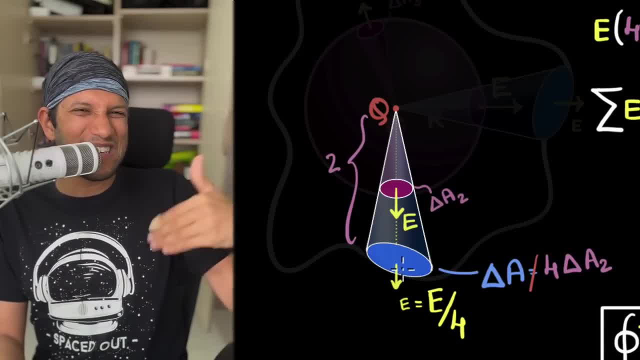 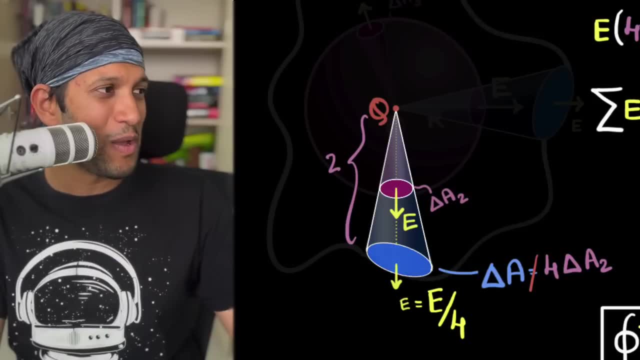 cone. it's just creating some crooked shape over there. it's like a truncated cone, so it won't work. What's the point, Feynman? Why are you wasting our time? But Feynman says: wait a second, instead of taking this blue piece, what if we considered a piece that actually completed? 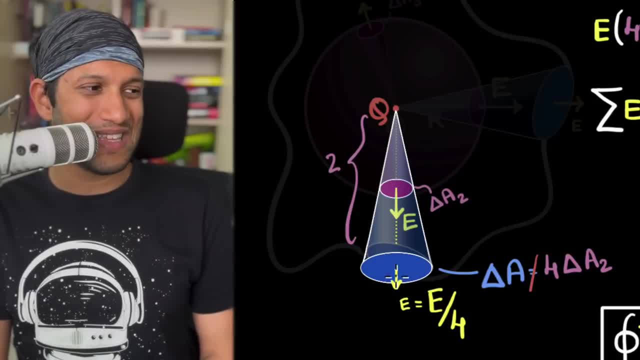 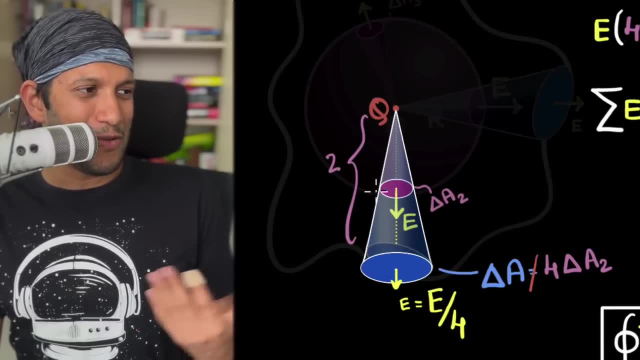 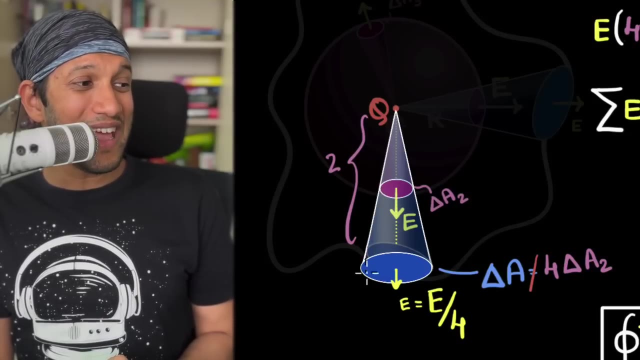 that cone very nicely, Now look. he says. now look, if we have a perfect right circular cone, then because of you know similar triangles, equivalent triangles, whatever that is, if this is twice as big as this distance, then this length, their diameter, will also be twice as big as this. 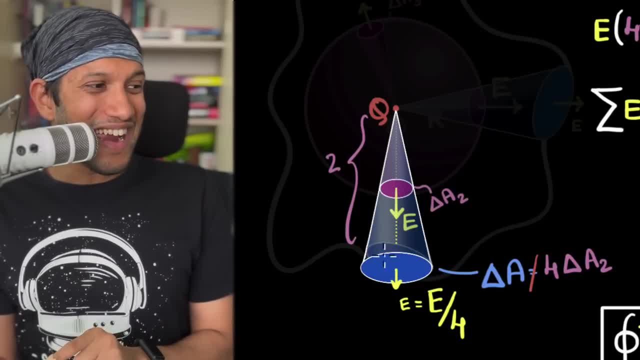 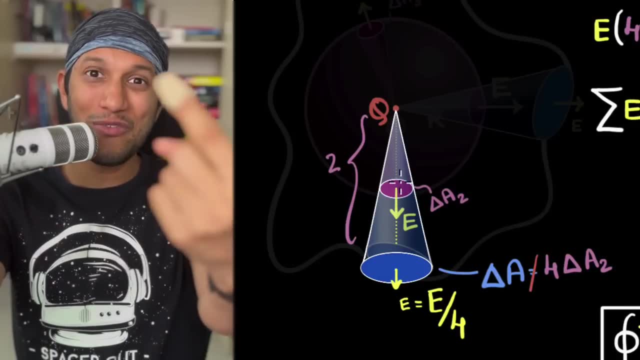 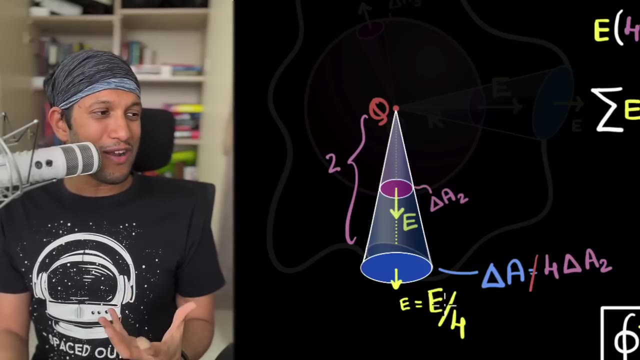 diameter, In other words, the area over here will also be not. also, area over here will be four times as much as this area, because area goes square of diameter, Which means if you consider this piece, then indeed it works out. the product of this piece will be four times as big as this area. 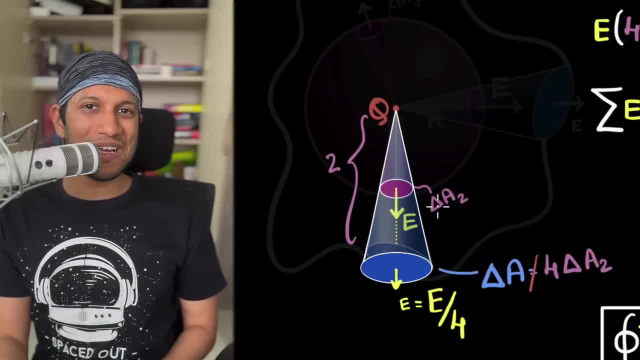 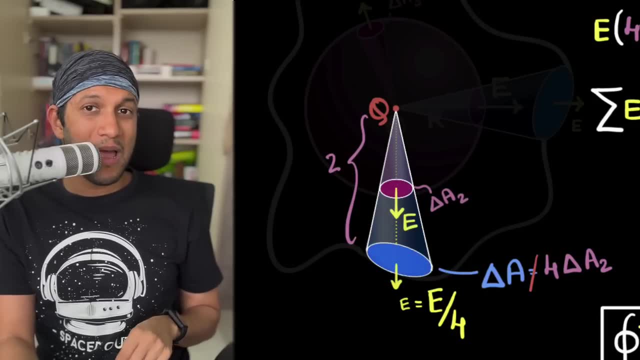 The product of eta and delta a will be exactly the same as the product of e and delta a. But I ask Feynman: but Feynman, what is that piece? That's not the piece that we are interested in. this is the piece that we should be looking for and Feynman says: Mahesh, what exactly is this piece? This piece? 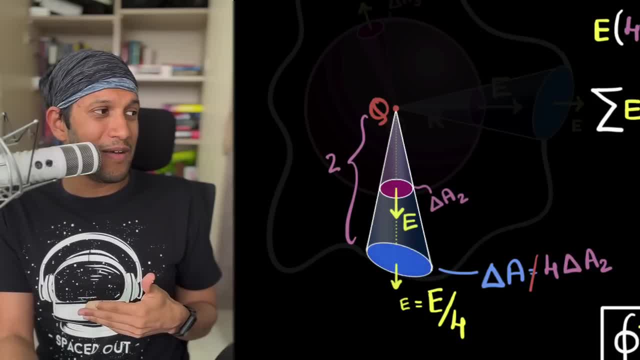 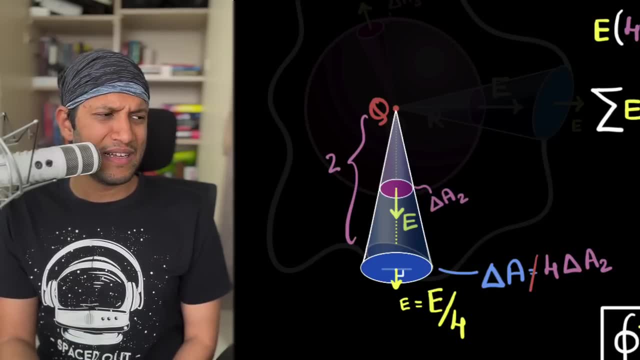 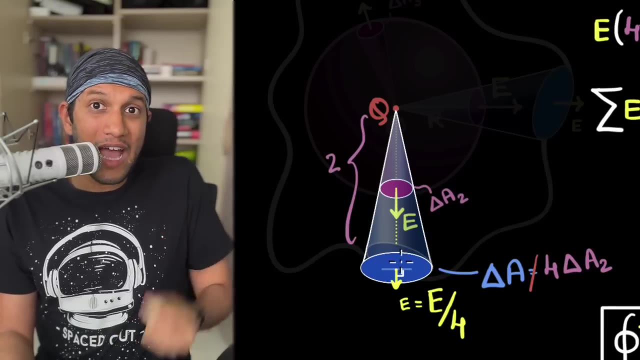 is actually the component of this area in the perpendicular direction to the electric field. That's what this piece is right. Yeah, so this means, Mahesh, you're right. if you take e into that earlier area, the actual area, it won't work out. but instead, if you multiply. 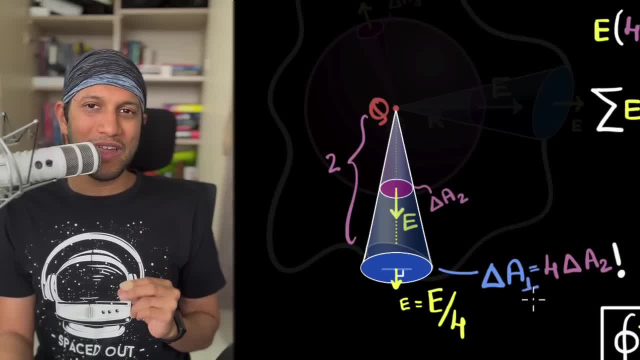 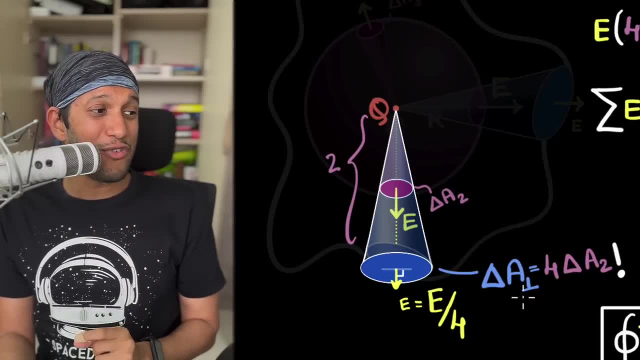 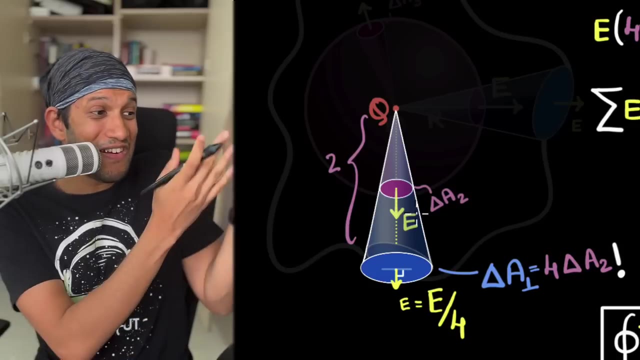 if you consider e into the perpendicular component of that area, it does work out. The perpendicular component does become four times as big as this, and if you take this product, indeed, it becomes the same as this product. Therefore, Feynman says: let's consider this product instead, Even here, for 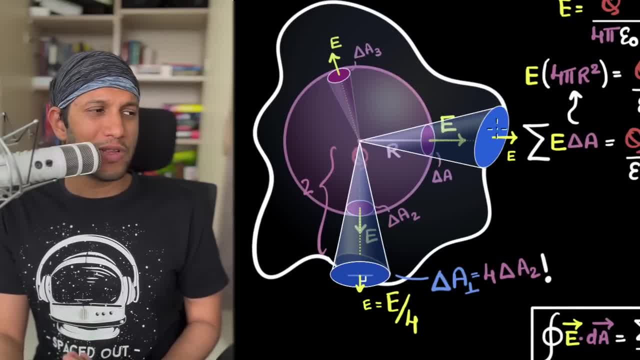 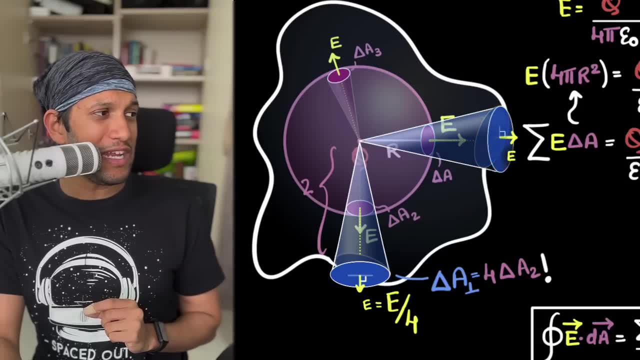 example, if you multiply e into the perpendicular component of that area, it does work out. But if you take e and delta a of this actual area, it will not be the same as e and delta a of this area will not be the same, But instead, if we consider the perpendicular component which forms the nice right circular cone, 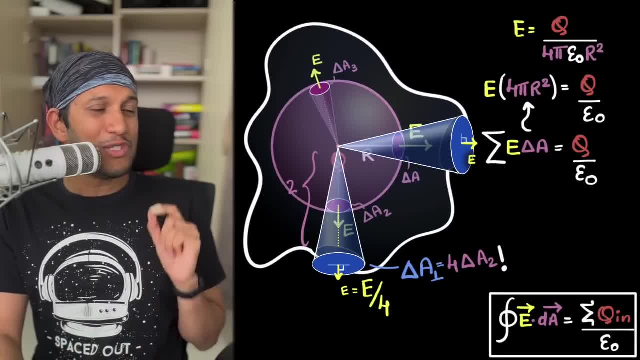 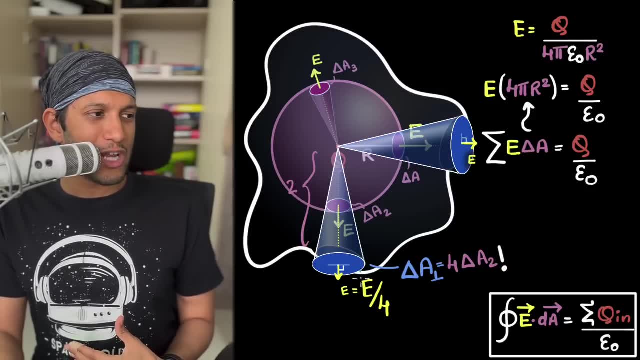 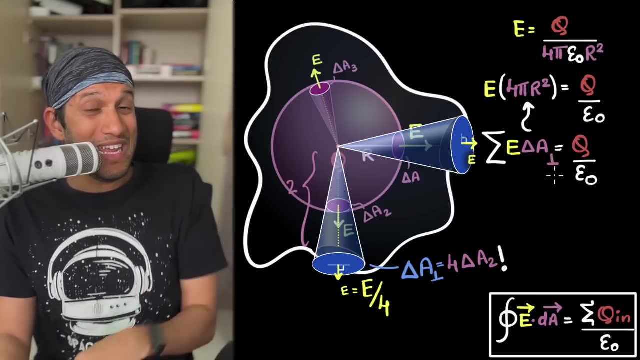 then that works out. That means we need to make a small modification. Feynman says: yes, I misspoke earlier. if you take e times delta, a of the actual pieces, it won't work out. but instead if you take e dot, e times delta, a perpendicular. 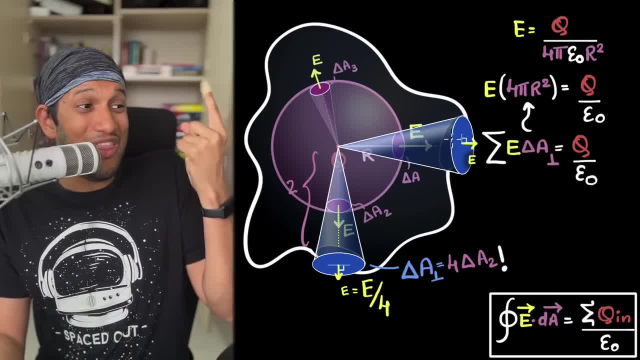 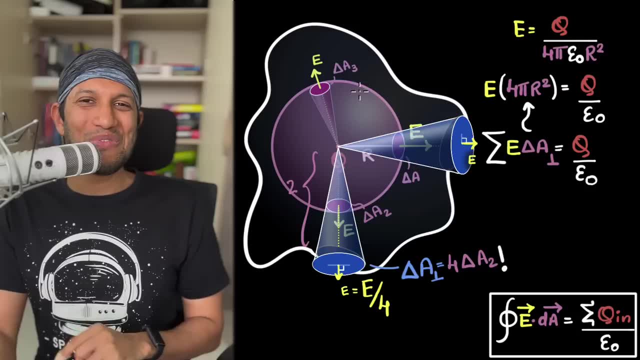 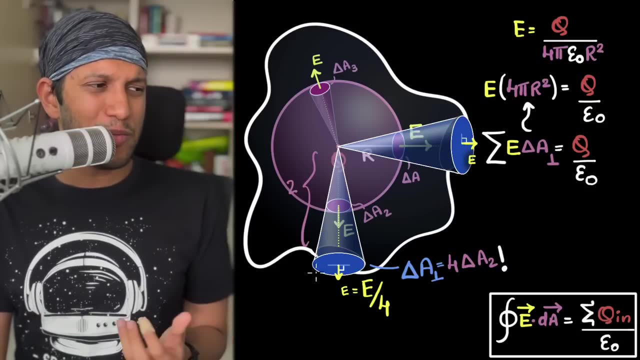 this is the perpendicular component to the electric field. if you take that piece, then it will indeed be equal to four e times four pi r squared. and so let's consider, that is what he says. and, of course, a small detail is we shouldn't be taking big areas, we should be taking very tiny, infinitesimal areas. 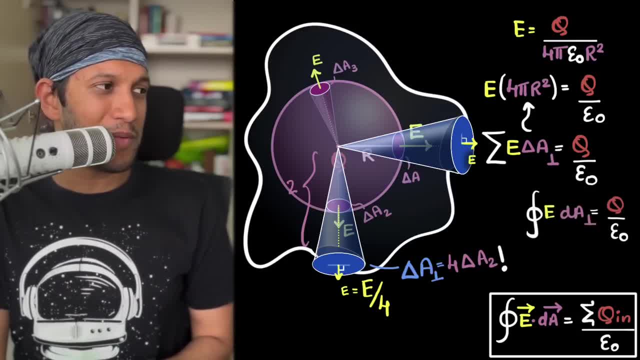 so this will become a, d, a and the whole summation becomes an integral. but we've, but we've got it. all we are saying is that if you take e and multiply it with the perpendicular component of the area at that location and add it all up over the entire surface, then it doesn't matter how big that surface is, what the shape or the size is, it will always equal q divided by epsilon. not why? because of this, just we saw. that's the intuition for it. that's the crux of Maxwell's equation. isn't that beautiful? just look at that, that's beautiful. 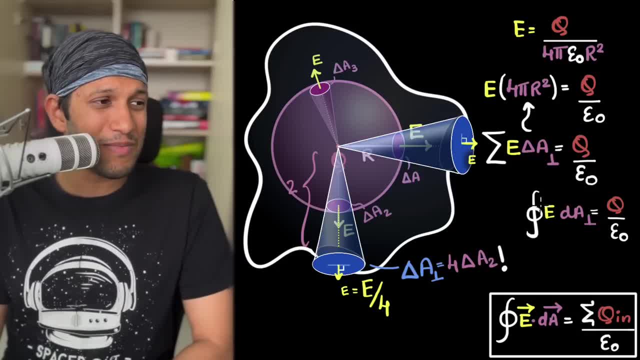 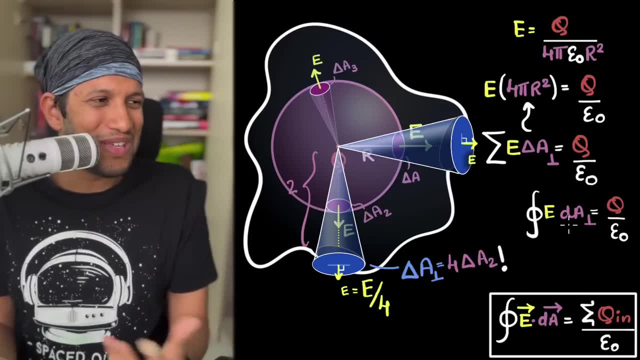 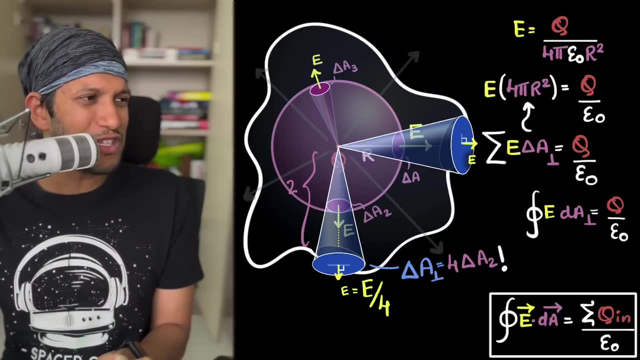 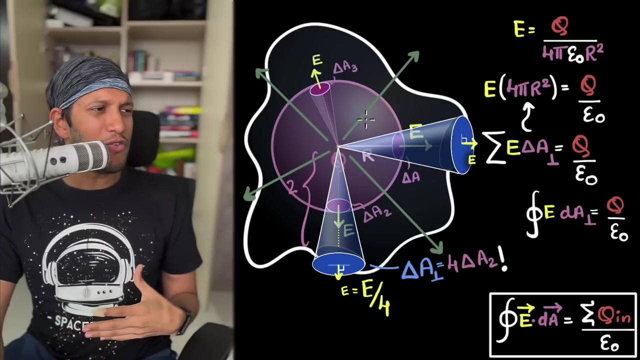 Now, at this point we should ask Weinmann: well, but why does it turn out to be like that? what is that? e into d? a perpendicular? it's so beautiful, isn't it? and Weinmann agrees it is so beautiful. in fact, it has the properties of something that's flowing outward. think about it: if you had a tiny sprinkler over here that's spreading out water, then the amount of water that goes out of this sphere would be the same as the amount of water that goes out of this sphere. 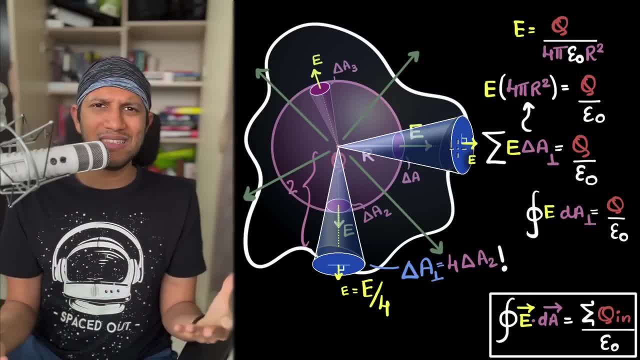 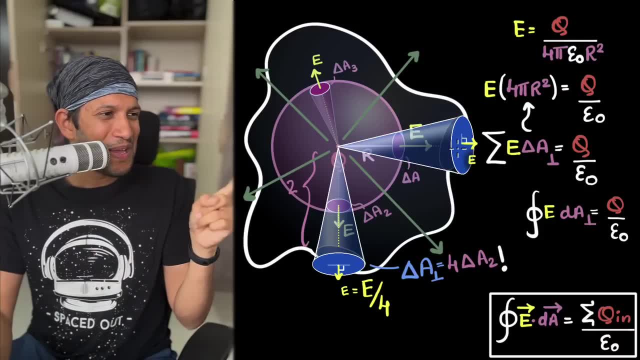 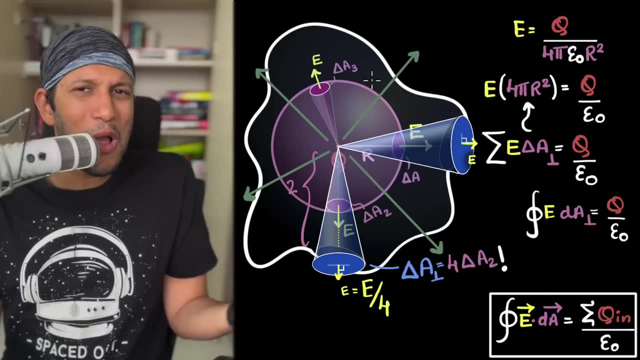 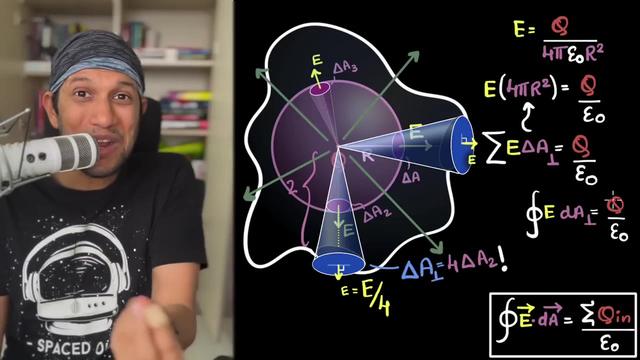 In fact, the amount of water that goes out of the sprinkler has nothing to do with what surface you choose here. that's something to do with only the sprinkler. how, the strength of that sprinkler- isn't it something very similar happening over here? this product, whatever that is, it has nothing to do with the surface that we are choosing. it has only something to do with the strength of that sprinkler, the sprinkler being the charge. so in some sense this product behaves very much like a sprinkler. 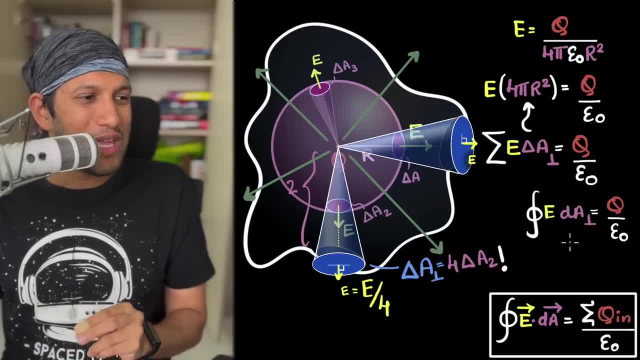 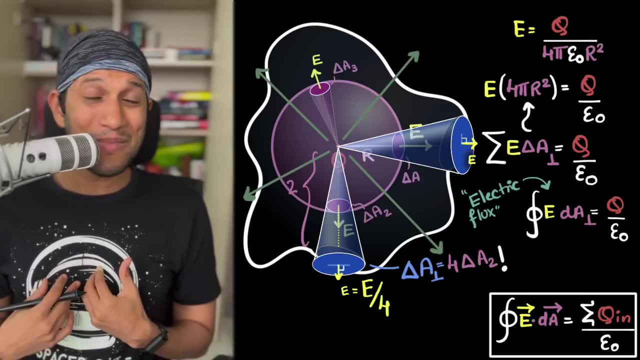 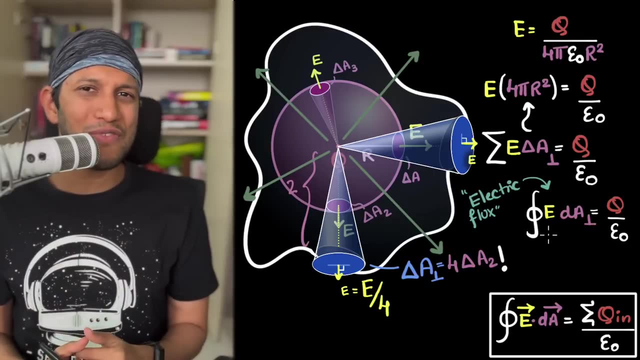 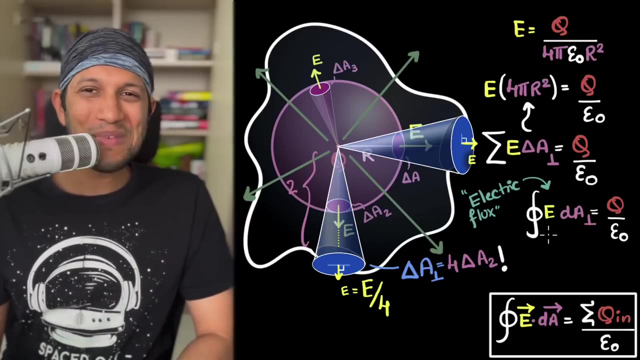 It behaves very much like something flowing. therefore we give it a name. we call it the electric flow or the electric flux. for a long time, I never understood why we define electric flux in the first place, why we define it as e times the perpendicular component of an area. but now it makes perfect sense, because it's that product that behaves like a flow. it's amazing, isn't it? all the hard work is done, folks. now we just have minor things. 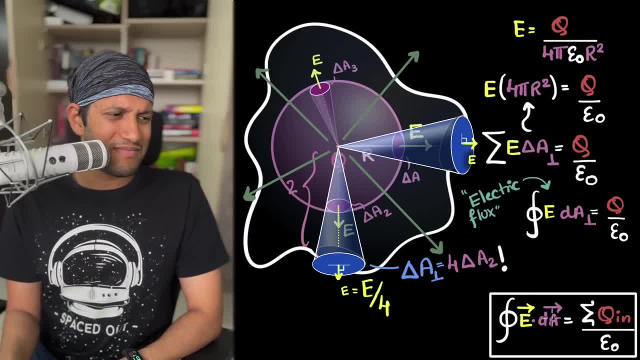 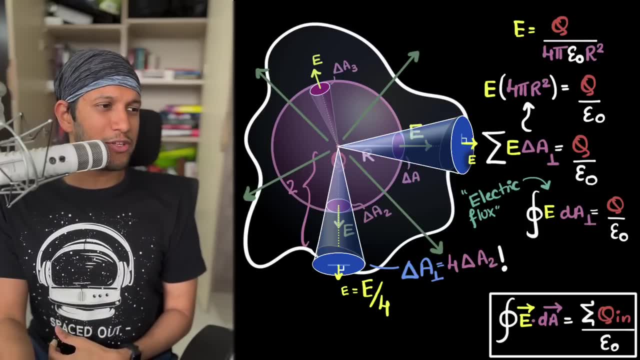 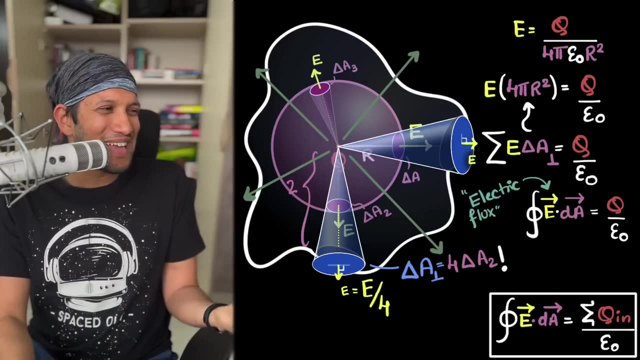 First thing. Second thing is: we might ask Feynman: well, what exactly is this dot? and there's an arrow mark over here. and Feynman says: well, it's the same thing, don't worry too much about it, it's just a fancy way of writing it. mathematicians like to write it in a fancy way and just call it e dot, da, but it's the same thing. it just means you take the electric field, multiply it with the perpendicular component of the area, but it's the same thing. all right, let's just write it in that fancy way. 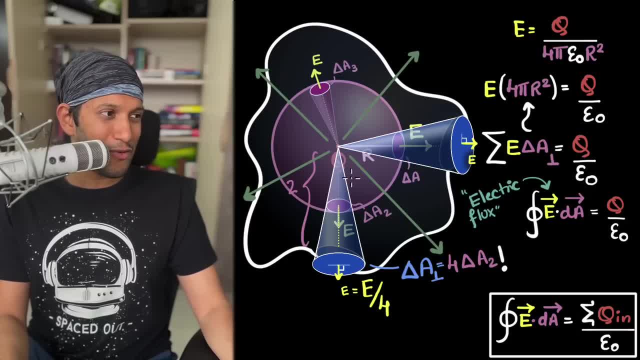 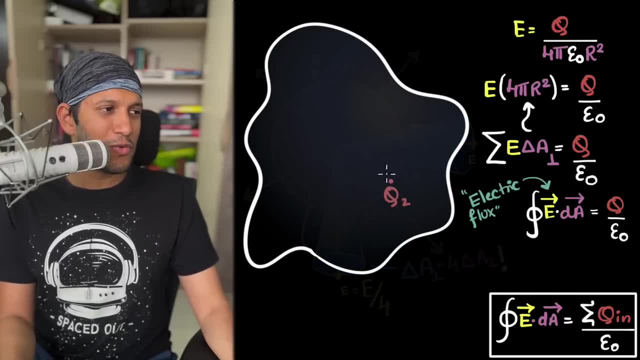 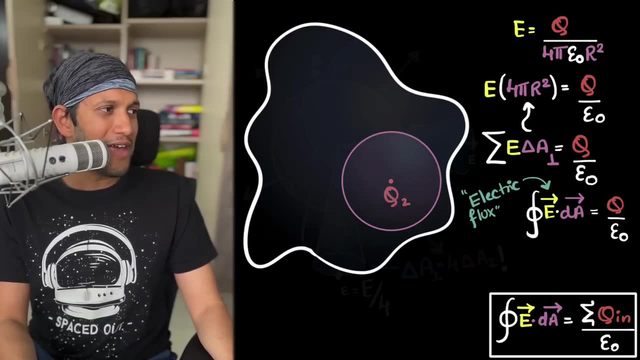 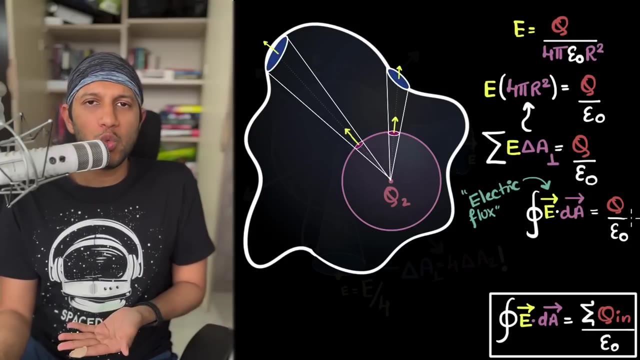 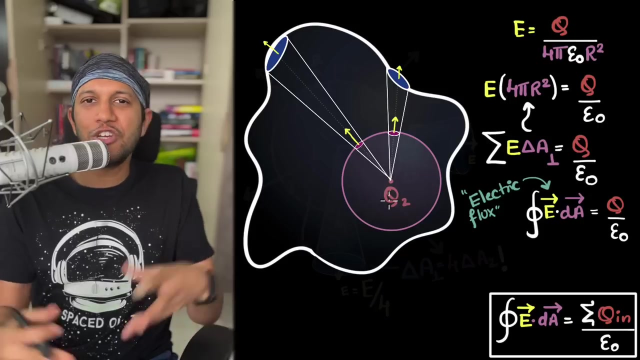 Secondly, what if you have another charge over here? Feynman, we have only considered one charge. well, Feynman said: let's consider it on your own, We're just that charge for a while. if I want to know what's the flux through due to this charge, through this entire surface? we do the same thing as before: we're going to draw a surface, a sphere, over here, and then we make all the argue, same arguments that we did, and therefore the flux due to this charge will be q2 divided by epsilon naught. and therefore, what would be the total flux due to this first charge and the second charge together? hey, it's going to be just q1 plus q2.. 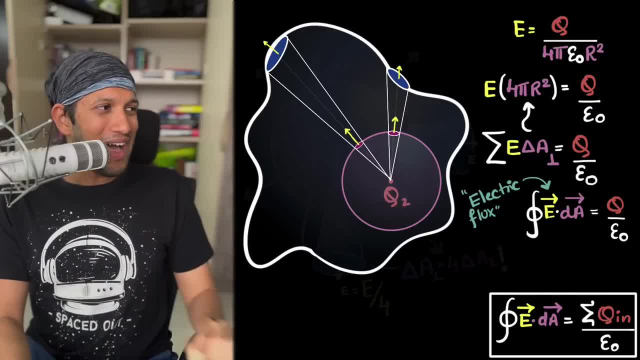 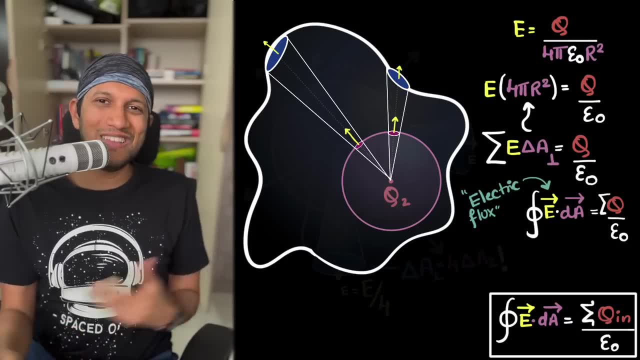 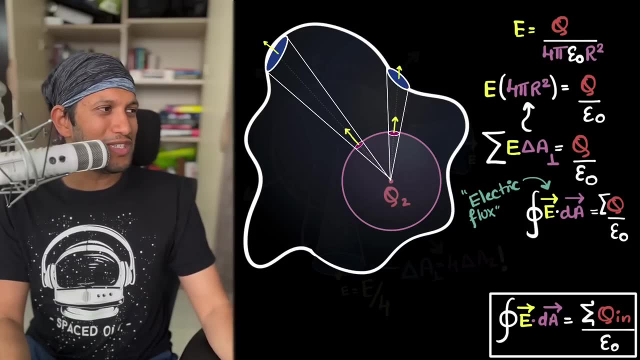 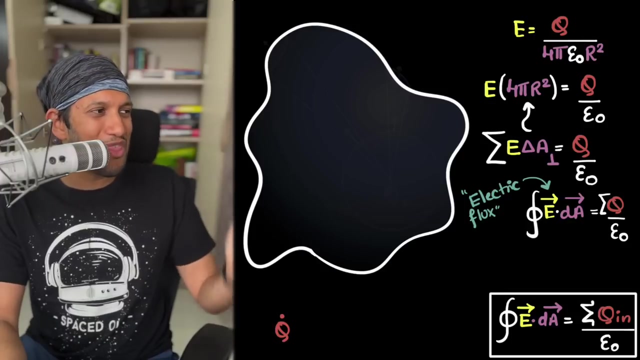 q2 divided by epsilon naught. that's why we write that the right hand side is the sum of all the charges that we find. but one last question we ask, Mr Feynman, is what if a charge is on the outside? what happens then? well, Feynman says: we've done all the hard work, let's use the same thing. if we draw something very similar to before, this time we're going to use the same thing. 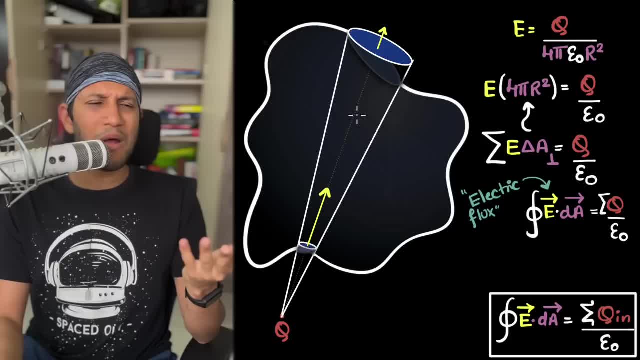 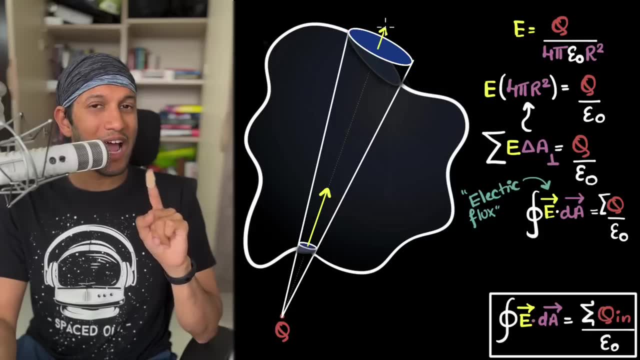 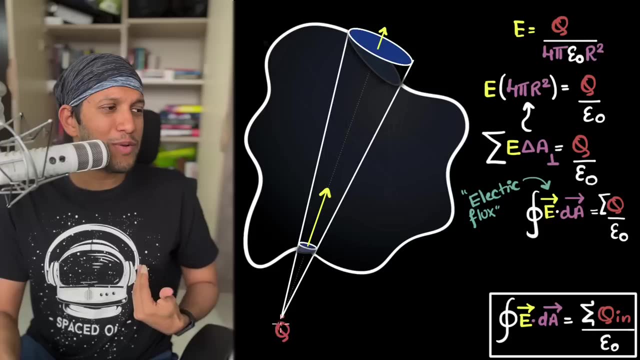 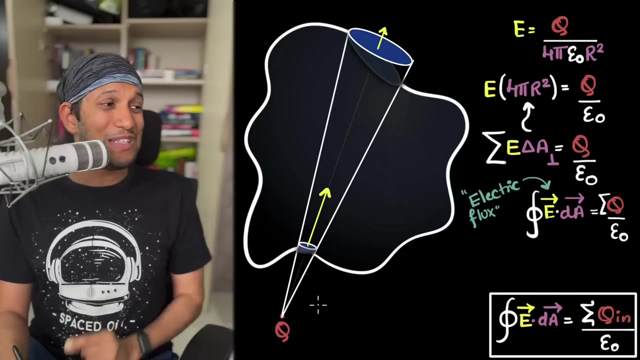 Again, you find the flux here should be the same as the flux here, same argument of the electric field and the area thing. but here there's an inward flux and here there's an outward flux. they're both equal, which means the net flux becomes zero. in other words, this does not contribute to any net flux, and I can do the same thing over the entire surface and therefore if a charge is outside, its contribution to the total flux is zero. it doesn't contribute at all because 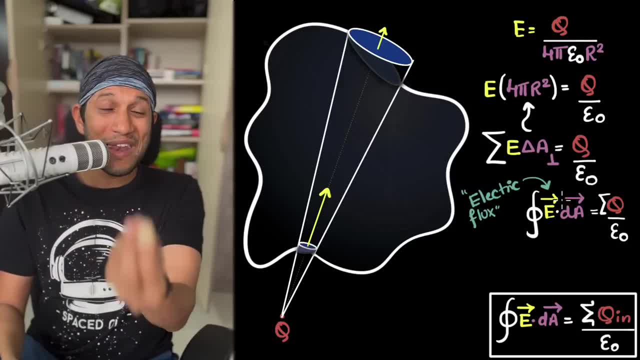 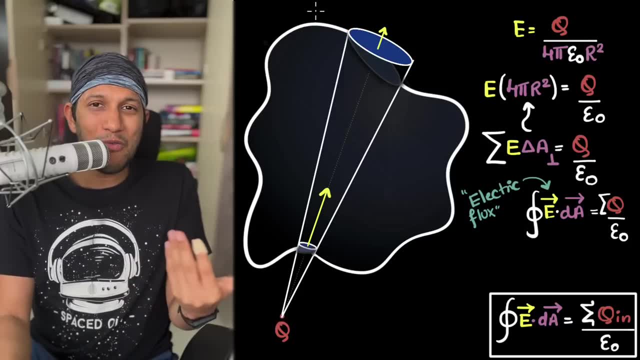 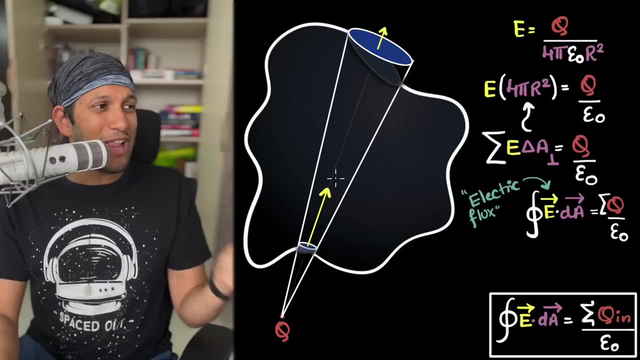 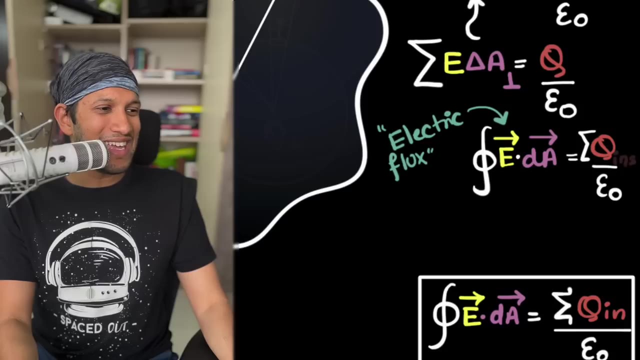 whatever inward flux it gives, it gives the same amount of outward flux. and look, the sprinkler does the same thing. if there was a sprinkler over here sprinkling water, whatever water enters, the same amount of water exits. so the net water that exited due to that sprinkler is zero, which means when you are calculating the total for sort of flux, what matters is only the charges that are on the inside. and there we go. in its full glory, the 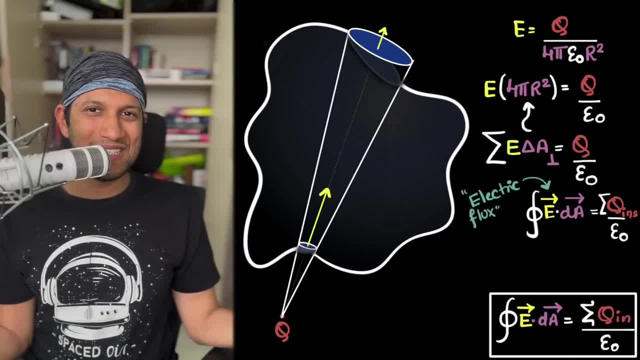 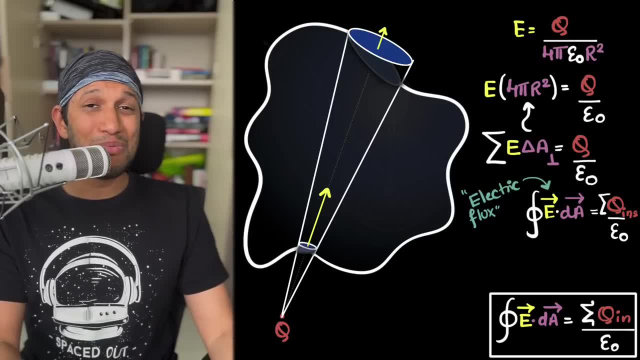 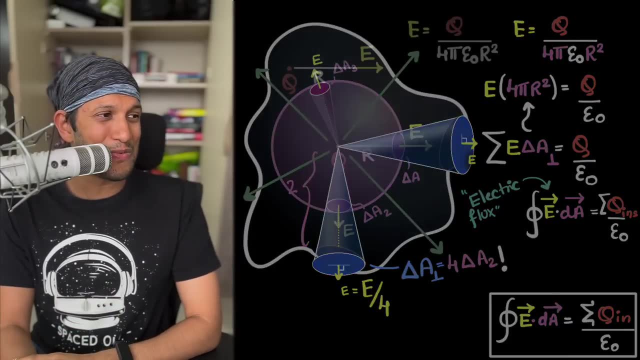 Maxwell's equation. we have it. we have it. we've derived it from Coulomb's law, but, more importantly, with pure logic, pure intuition and some brilliant arguments. well done, Feynman. well done. it's time to apply this. Feynman. what was that problem that Newton was struggling with? well, Newton says: 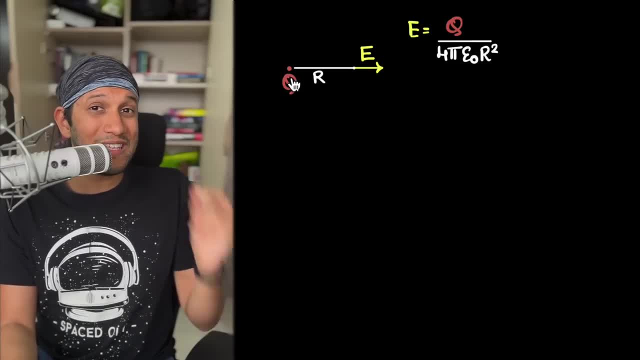 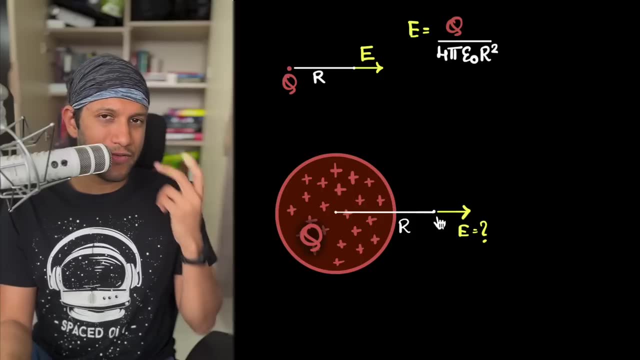 remember Coulomb's law. you know that Coulomb's law can be used for a single point charge, right? what if you have a ball of charge and you need to figure out the electric field at some distance are outside of it. how do you calculate that? well, my first instinct is: can I just use Coulomb's law? 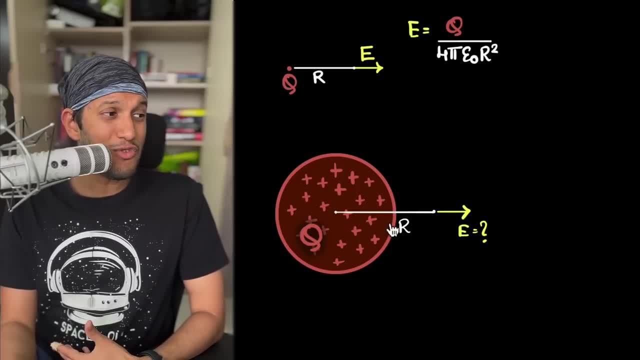 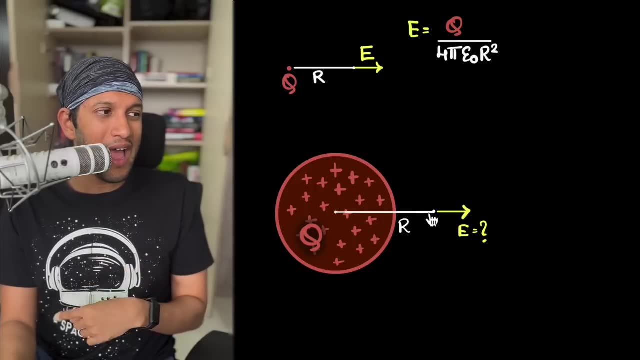 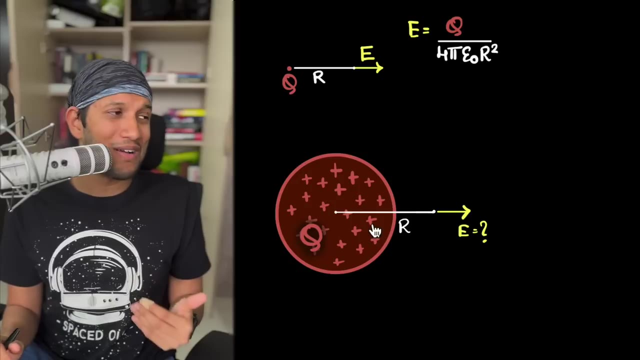 oh no, because it only works for a point charge. so if you have to actually calculate for the whole ball of charge, you have to take a very tiny piece dq, calculate the electric field due to that and then integrate over the entire sphere. and let me tell you that integral is nasty: it's pages long. 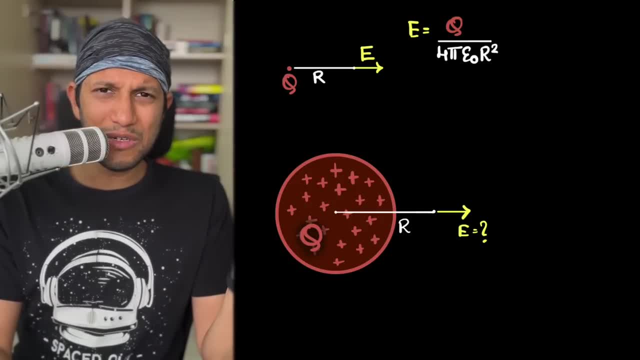 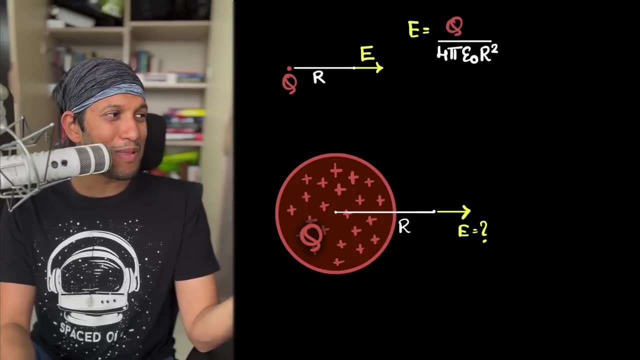 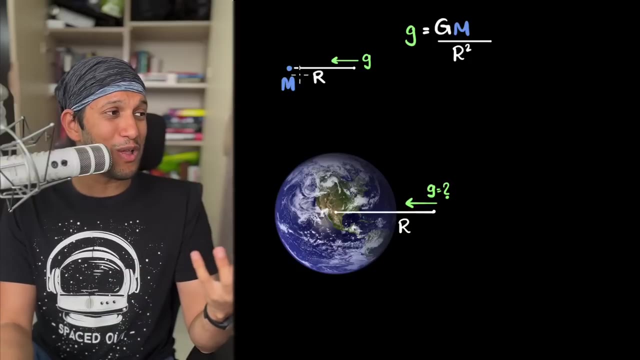 and I'm like, wait a second, is this what Newton was struggling with? why was Newton struggling with this? well, Feynman says silly no, not on this problem, but a very analogous problem. he was trying to figure out the gravitational field due to earth. see, just like with Coulomb's law, Newton's law. 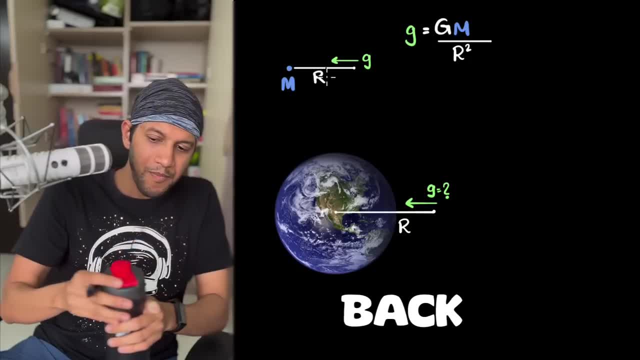 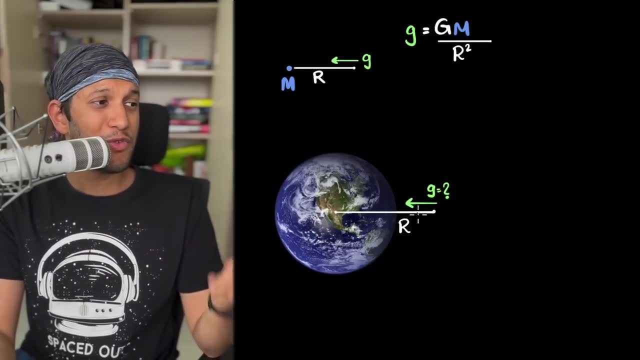 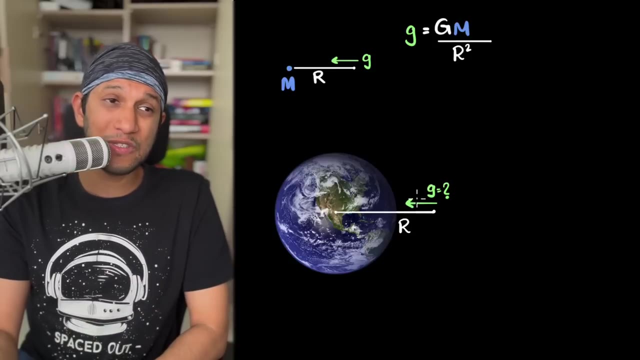 you see, just like Coulomb's law, the Newton's universal gravitational law only works for point masses, which means if you have to calculate the field gravitational field close to the earth, you have to do the integral. and that's exactly was Newton was struggling with for years. he did the integral. it took him years, he. 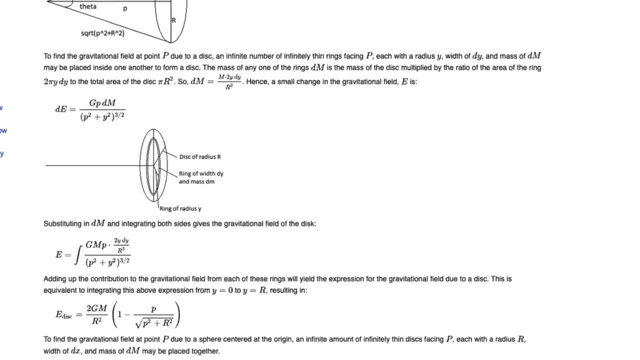 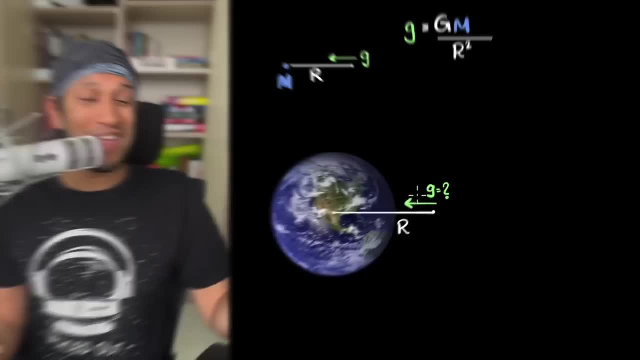 eventually did it, though of course he himself invented calculus, by the way, and he did it, and that was a nasty proof and whatever that is, he did it. but we can do the same thing in minutes now, or maybe in seconds- actually minutes. so let's go back to our problem. I mean, it's the same problem, we'll. 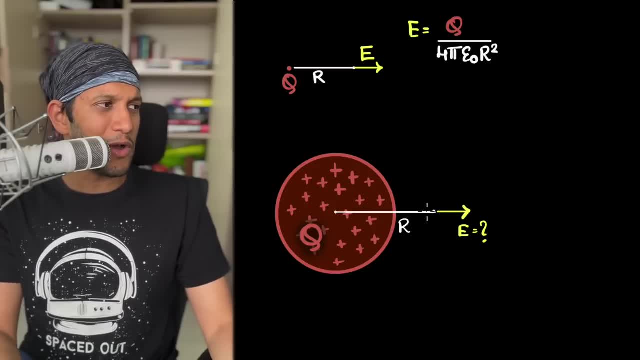 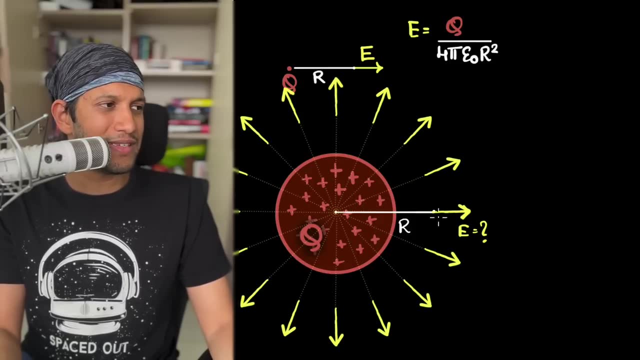 do it for charges, because we're working with charges, all right. how do we figure this out? well, the first step is to understand how to do it for charges. so let's go back to our problem and understand the symmetry. because of the spherical symmetry, the electric field everywhere at the 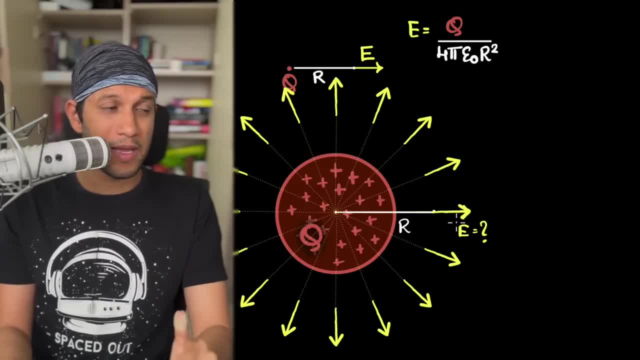 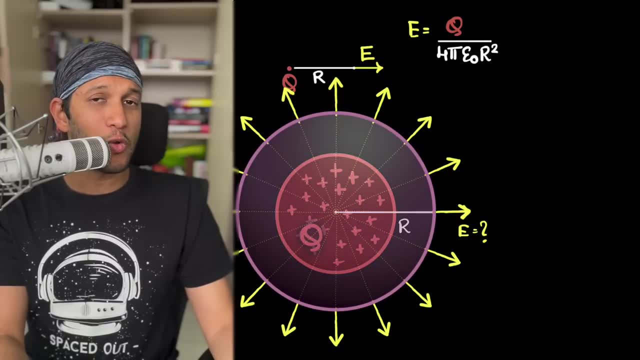 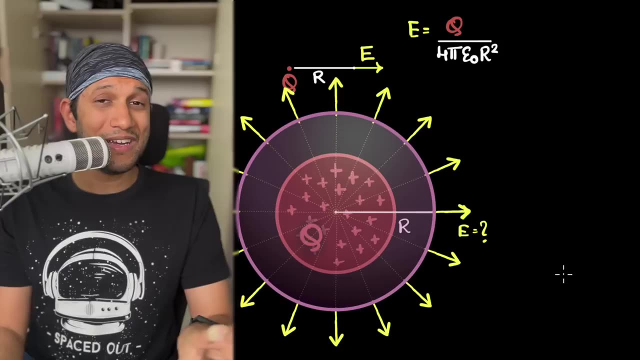 distance r will be exactly the same and radially away. because it's a sphere right and because of the symmetry, what we do is first we draw a closed surface. this is also called a gaussian surface because maxwell's first equation, all the things that we do we did- was first done by carl frederick. 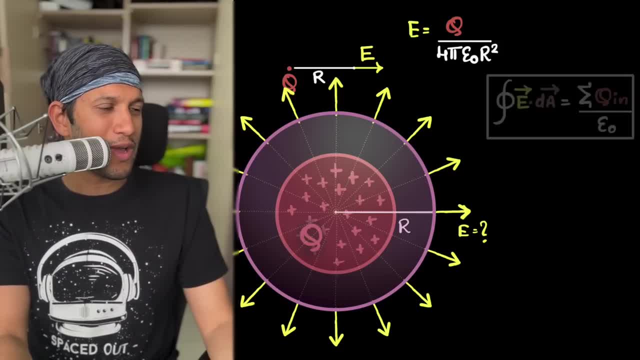 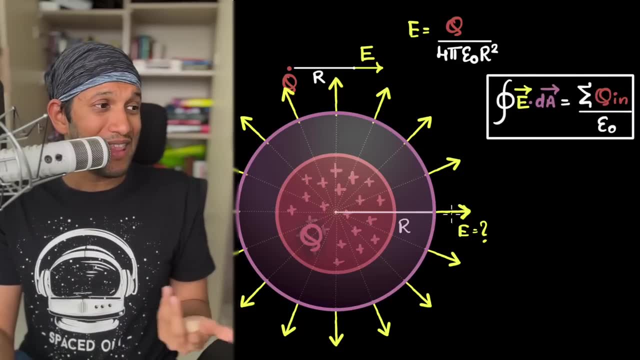 gauss. so we draw a gaussian surface and now we look at the maxwell's first equation, which is called gauss's law, as well. what about the left hand side? remember the left hand side, because we have a sphere. we have to figure out the electric field multiplied by the tiny area over here. and 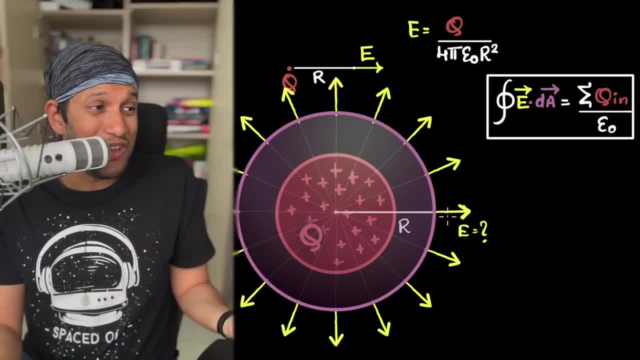 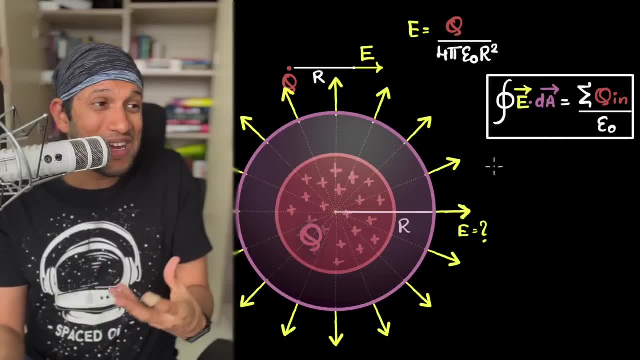 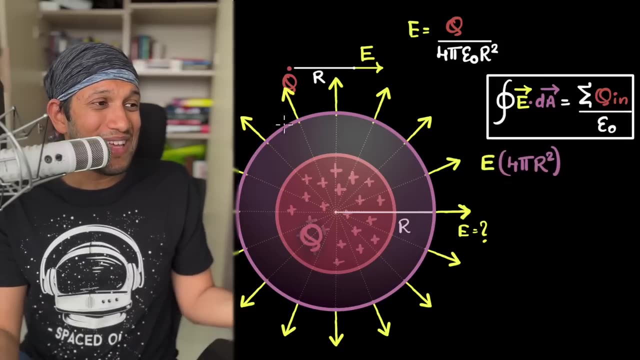 then sum it all up. that's what the left hand side is. but because this is a sphere, the electric field everywhere is the same, just like what we did before. the electric field pops out and all you get is the summation of all the areas. that is basically the four pi r squared, which means the left hand side just becomes e times. 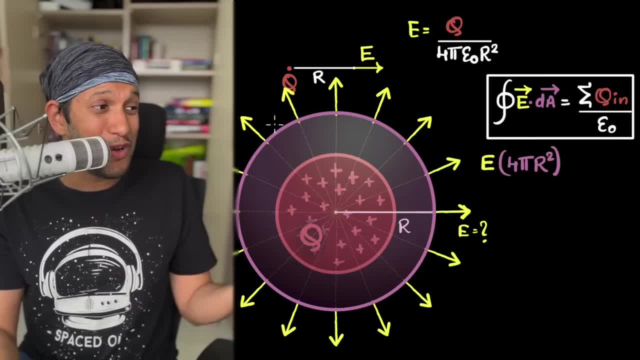 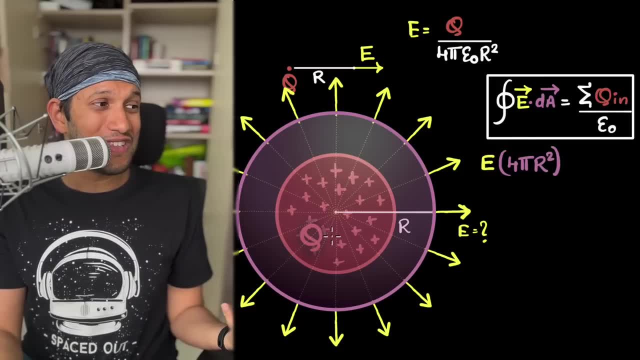 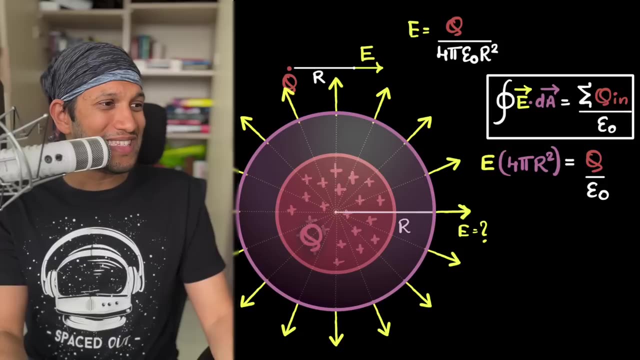 four pi r squared. so look, even though there's an integral over here, when you are using it for a symmetric case, that integral vanishes. what is the right hand side? right hand side is the total charge that's inside that gaussian surface and that charge is just q. and there you go. that means 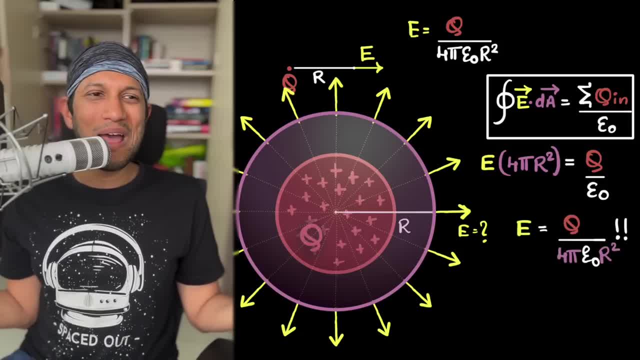 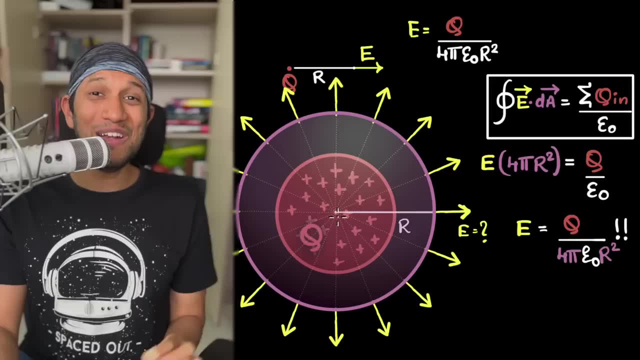 the electric field just happens to be q divided by four, pi, epsilon naught r squared, you get the sum of the total charge that's inside that gaussian surface and that charge is just q, same result as you get if you had a charge at the center of it. just imagine how frustrated newton. 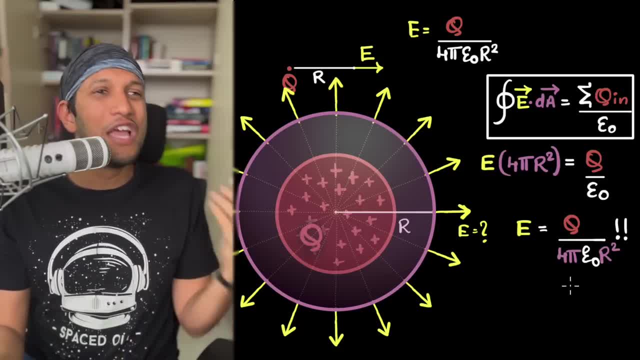 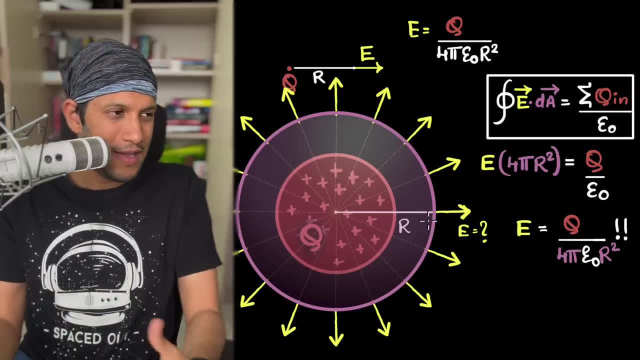 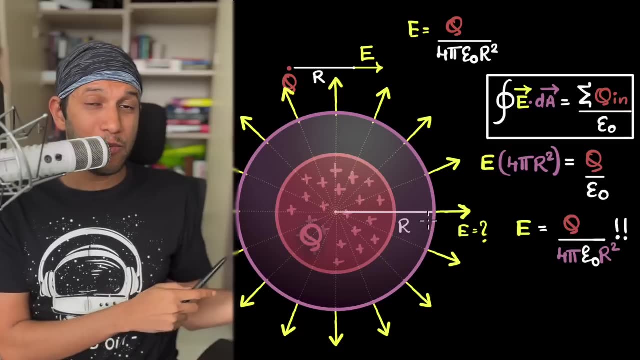 must have felt. after doing all that integral and everything, he gets the same result. fineman says well in his defense: newton already intuitively knew that the gravitational field should look very similar, but he just wanted to prove it mathematically well. so there's one way to prove. 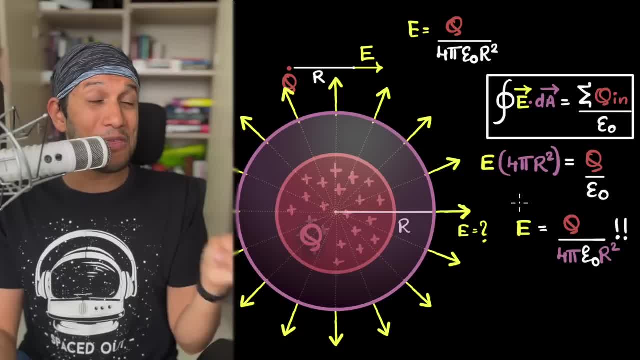 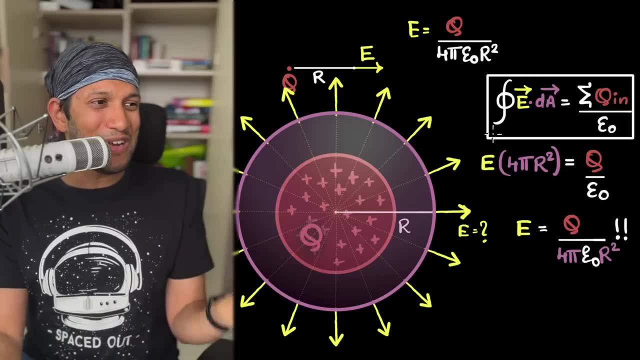 that you do all that integrals. but this is all you have to do: is you do all that integrals and also a rigorous mathematical proof. and what i find amazing is that we started with coulomb's law, but we took a different route. instead of integral, we went into this and created this beautiful 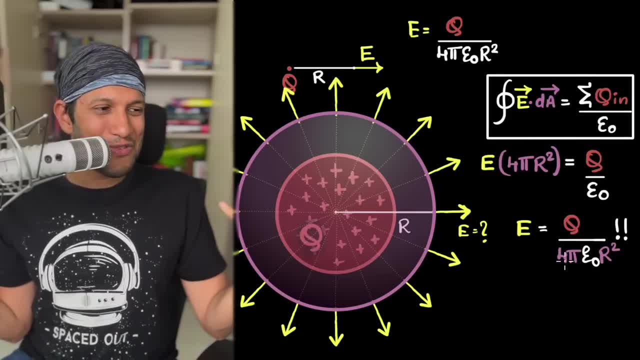 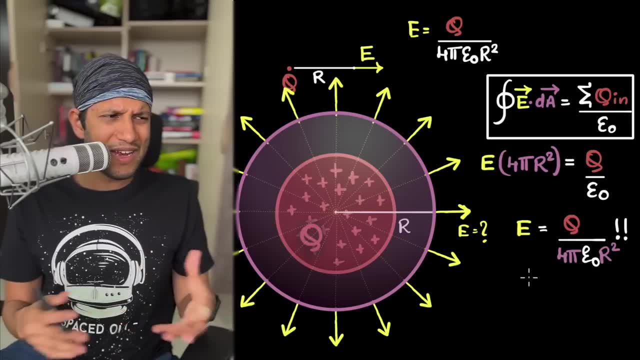 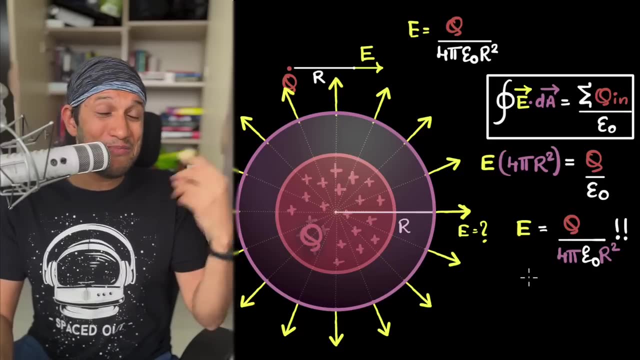 equation, and now we exploited that equation to then get the fruits of it, isn't that? i don't know? is this, this is amazing, whoo, all right, uh, fineman, do we have time for max for second equation, and it's already almost done? what? yes, you can just build up on this and we'll immediately get max. 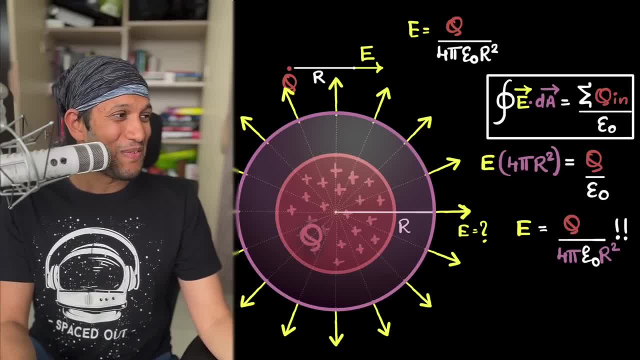 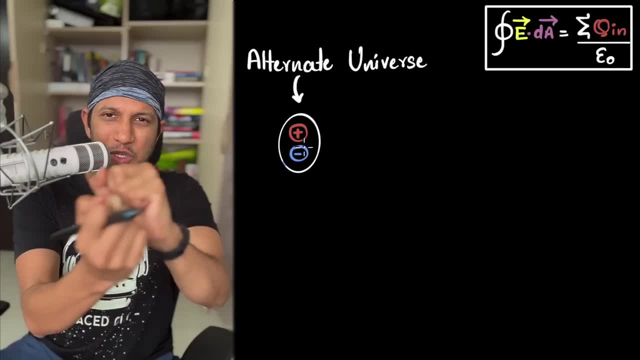 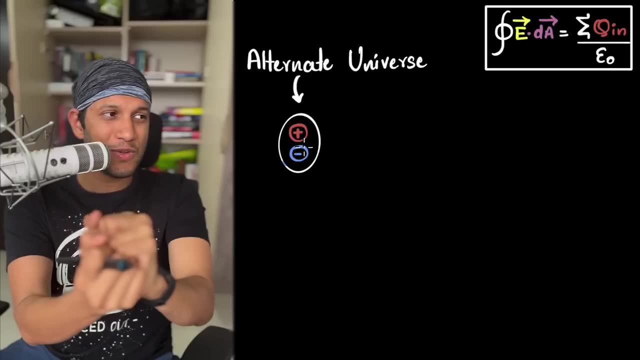 for second equation: all right, fineman, how do we do it? well, fineman says: for this: imagine an alternate universe in which we have positive and negative charges always coming together as a dipole. okay, if they were inseparable, if you always, always had positive and negative charges together and everything else the same. 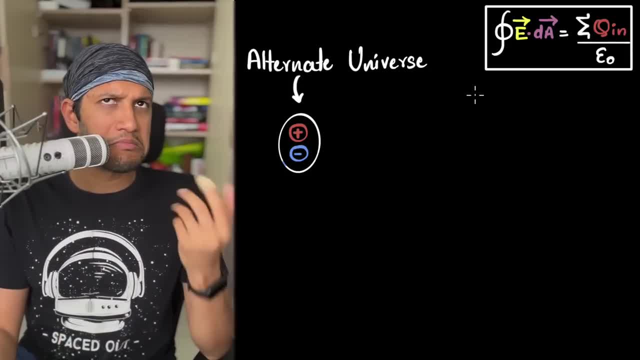 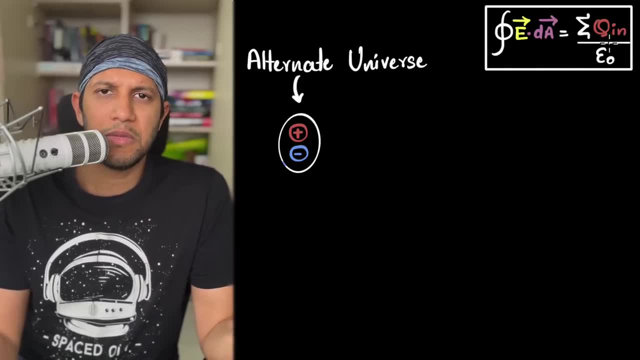 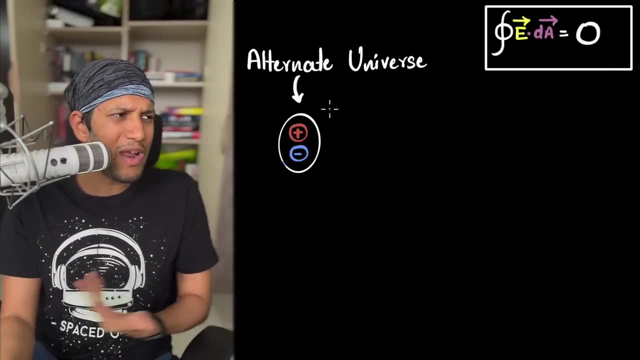 what would gauss's law look like in that universe? and i say: well then, whatever surface you choose, the total charge inside will always be zero, always having positives and negatives together. so total charge will always be zero. this is what the gauss's law would look like. but i asked: fineman, why are we considering alternate and hypothetical? 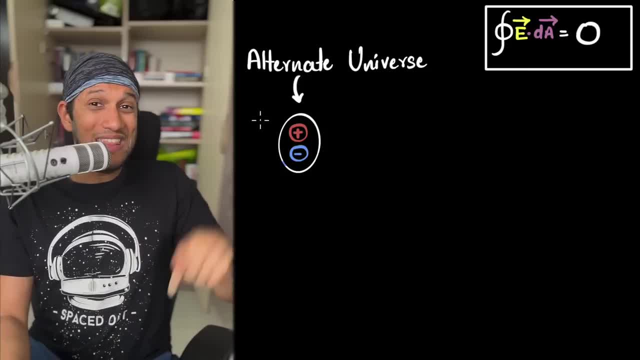 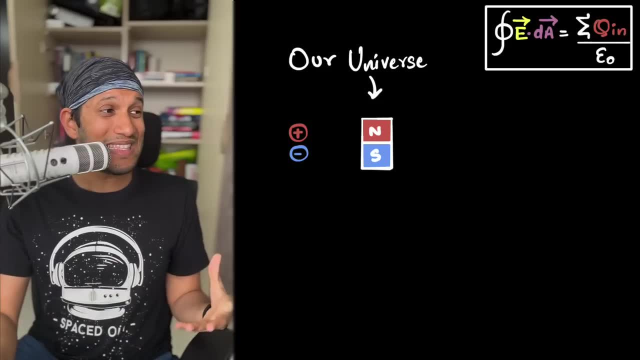 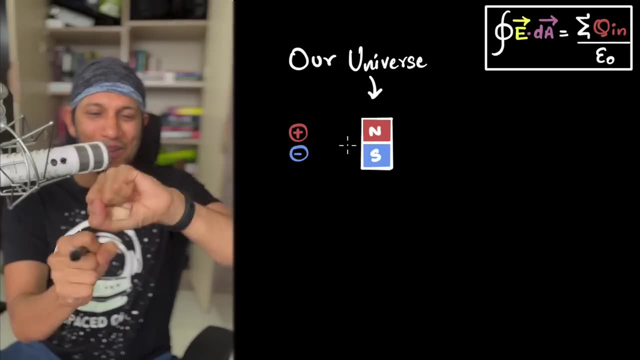 universes, because fineman says this is true in this universe as well, not for electricity, but for magnetism. he says that in magnetism, unlike electricity, you do not have a single north pole or a single south pole. north and south comes always together, and our first instinct might be: 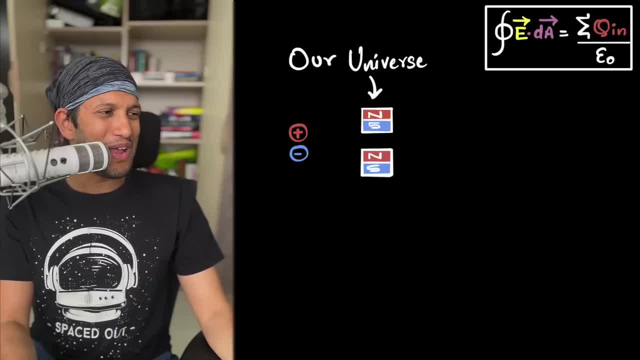 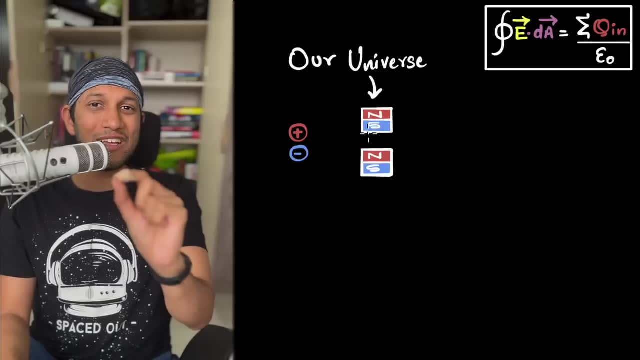 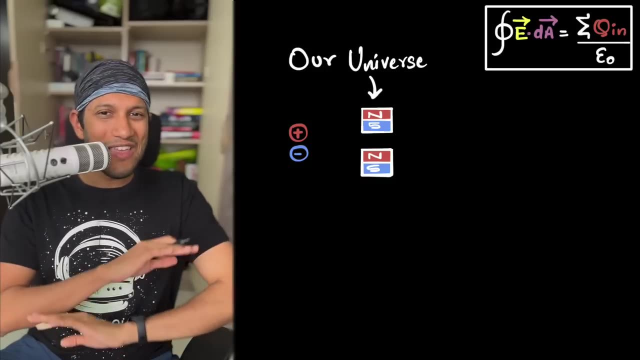 to just break the magnet. but we don't we. if we break the magnet, we'll again get a north and south, we'll again get a magnetic dipole. and even if you go down to the level of a single electron, it is a magnetic dipole. which means, if we were to now write down maxwell's second equation, i think you have. 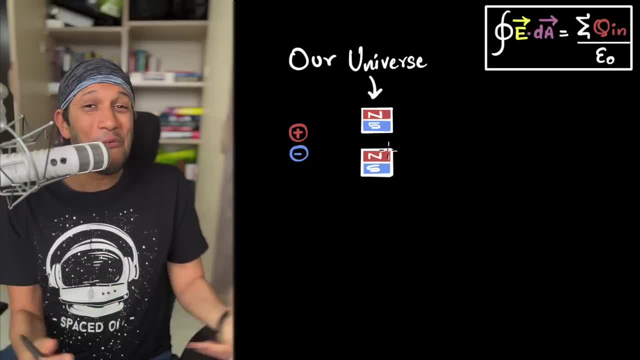 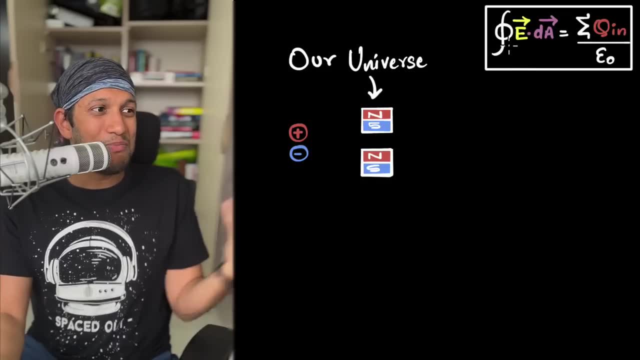 everything to everything you have. you should be able to write it down. what would maxwell's second equation be? come on, folks, i think we can do it. well, maxwell's second equation is basically the same thing for magnetism. it says that if you take the magnetic flux over a closed surface, 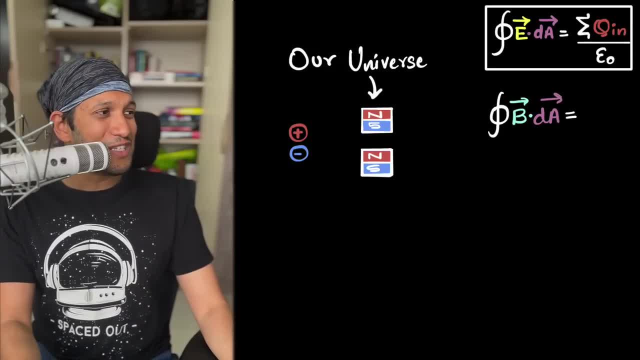 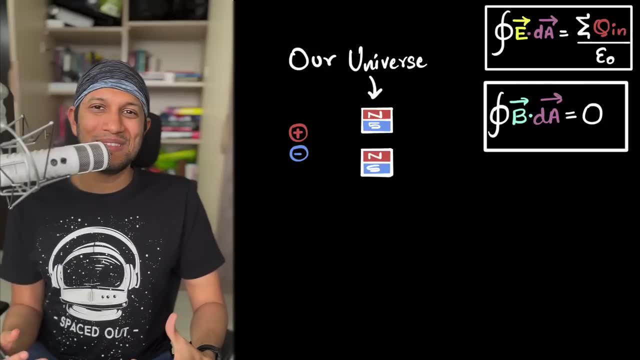 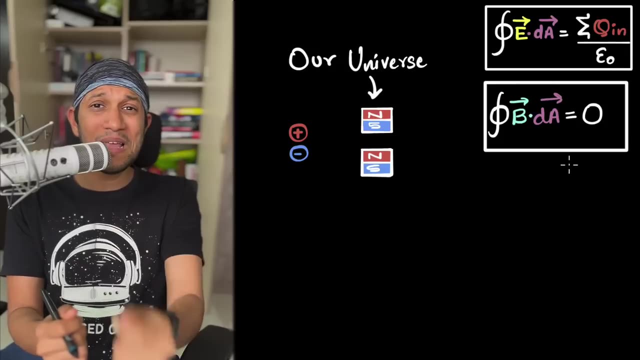 what should that answer be? it should always be zero, because you only have dipoles. so the maxwell's second equation is basically telling us that there are no such thing as magnetic monopoles, you only have magnetic dipoles. there we have it, two maxwell's equations. 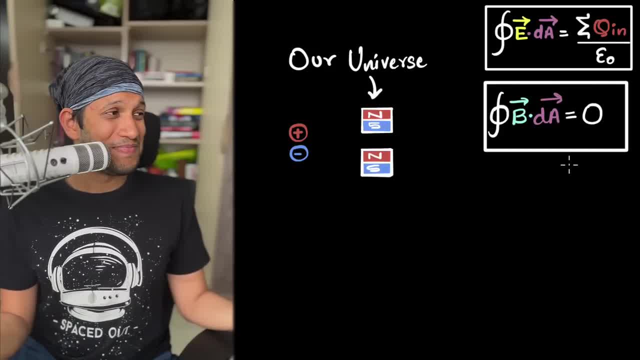 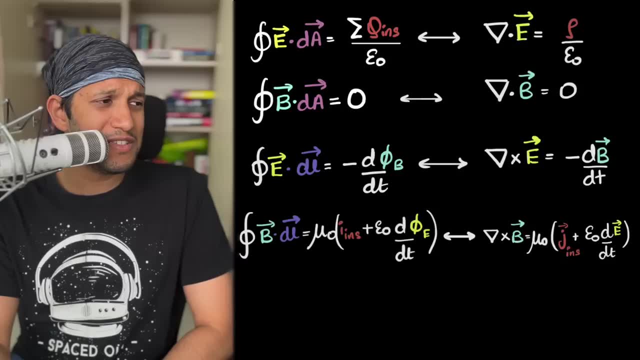 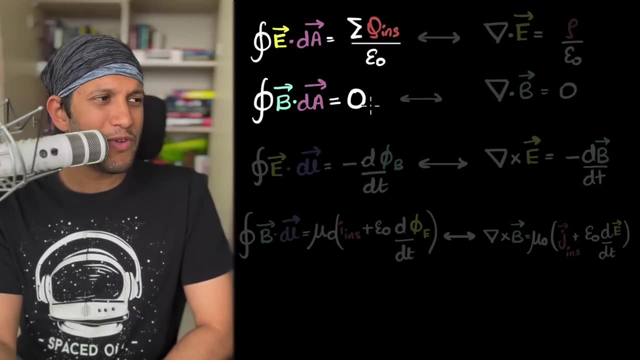 down, all by intuition. finally, before we end, we ask feinman. but, feinman, we still have a long way to go. what about these other monstrous looking equations? and he says, well, mahesh, the hard work is already done. we can use the intuition that we've gotten for these two equations and use that.